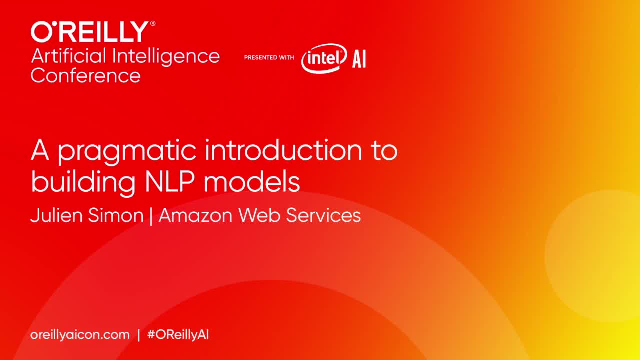 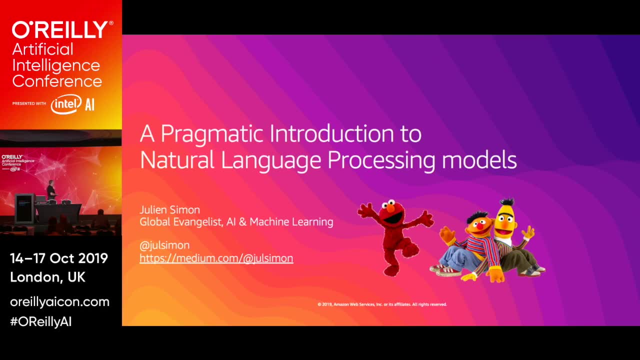 Thank you very much, Hi everybody. So, yeah, I guess the key word here is pragmatic. My goal today is really to give you an overview of the main NLP models and show you a couple of demos that hopefully don't scare you away, Because those animals here they look friendly. 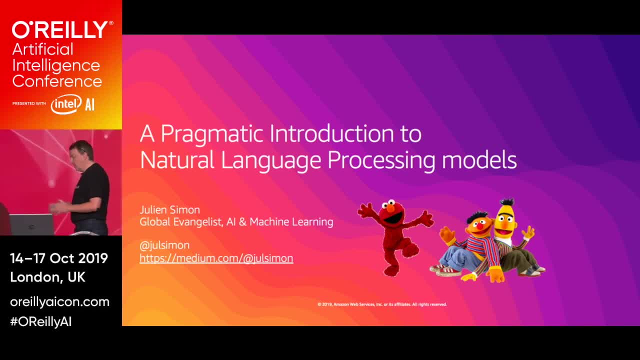 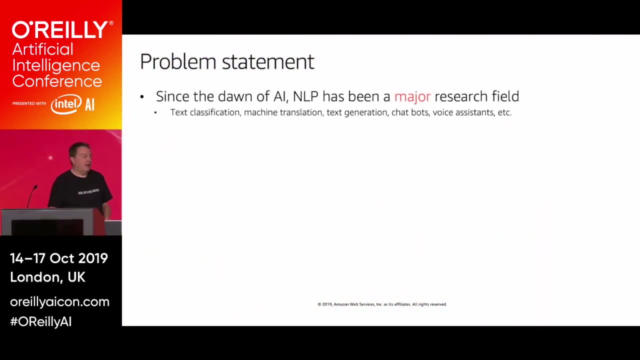 but they bite. So I really want to show you that you can get to work with these models- and some of them are absolutely state of the art models- without having a PhD or without being a world expert. So the problem statement is this: Of course, NLP has been around forever. 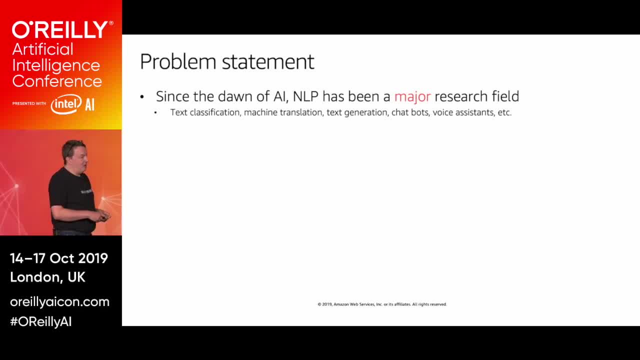 It's just as old as AI is, And well you know, there's been a lot of focus on computer vision and crazy CNNs for the last few years, and those are nice and fun, But NLP is at least as important because it lets us do things like text classification, translation. 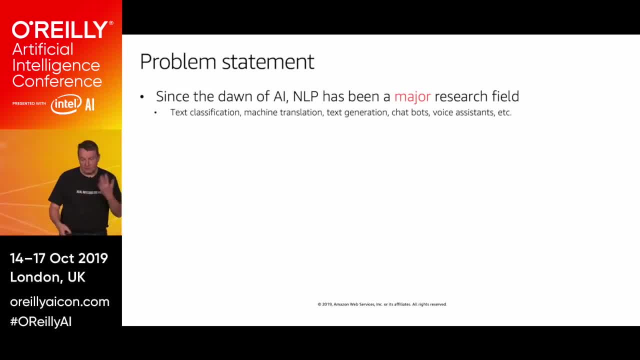 text generation, chat bots, voice assistants- everything That of course involves speech and language, which is very central to what humans are. So if we think we can build AI systems, then of course we have to think about how we integrate speech and voice in. 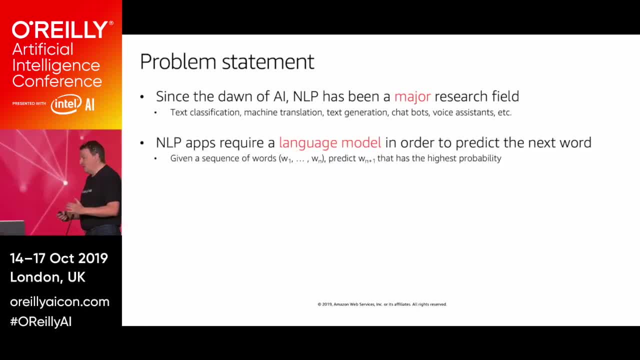 there. So the problem is this, Of course, text characters strings. these are meaningless to computer systems. We need numbers, We need vectors, We need matrices. So we need to build a language model that lets us predict what the next word should be. So, given a sequence, 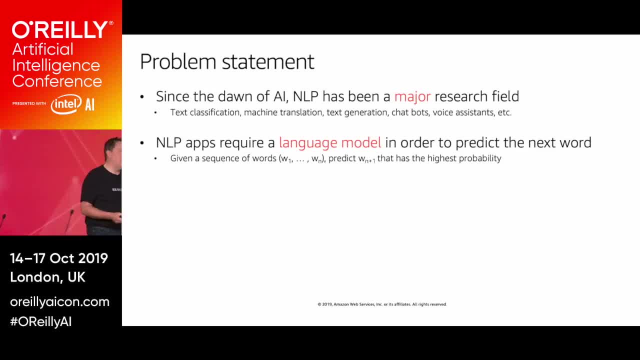 of words. Later today I'm going to take the train back to Paris, probably, Hopefully, if it stays on track. And that's exactly the problem we're trying to solve. We're trying to predict what comes next. Okay, And this is really the core of the problem we're trying to solve. 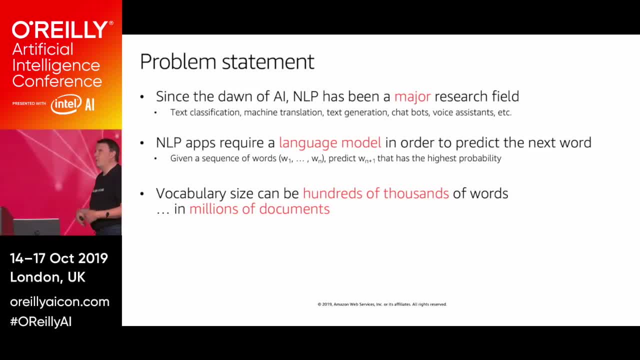 Obviously, the vocabulary- Or vocabularies, because of course we want to do this in different languages that we're dealing with- are huge, So you could argue that Most people around us seem to have 500 words of vocabulary, And it gets worse every day. 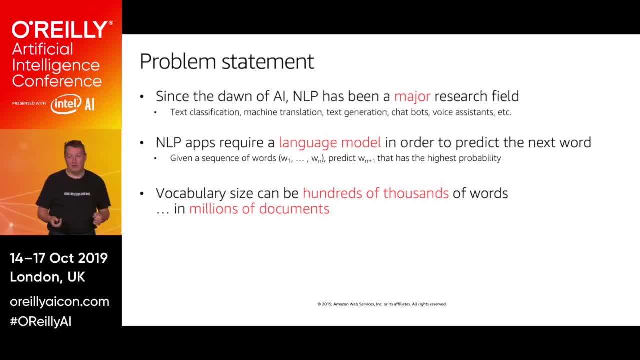 But in theory we should be able to use hundreds of thousands of words And we should be able to understand their context in millions of documents. So we're talking big corpuses here, Billions of words, Maybe tens of billions, hundreds of billions of words. Think Wikipedia. 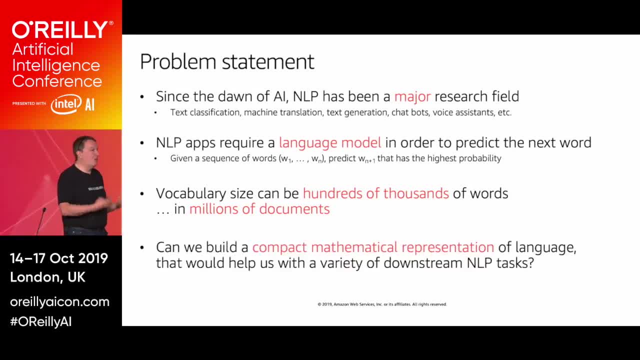 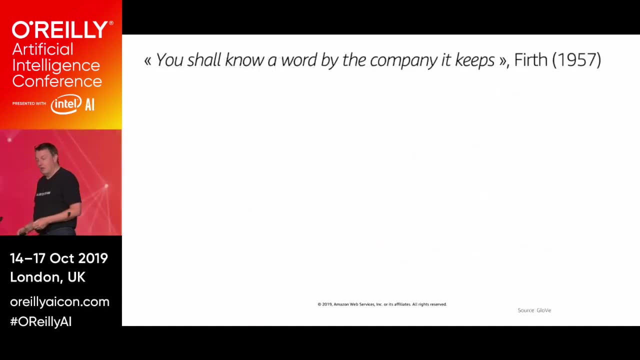 Lots and lots of data. So can we build a model, a compact mathematical representation of language that will help us with all those downstream tasks like sentiment analysis, classification and so on. So that's the basic problem we're trying to solve. Of course you've all seen. 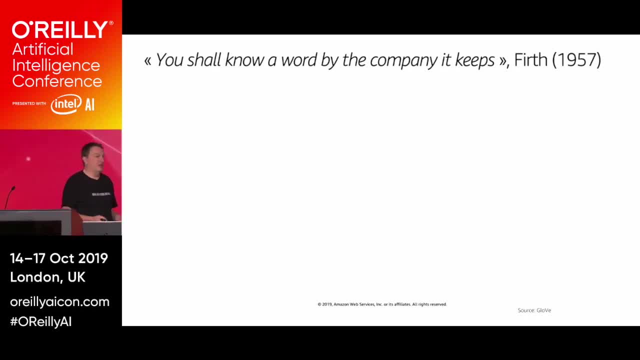 this sentence and this quote a million times, but it still is central, Right, You shall know, a word by the company that it keeps, And what it really means is if you want to understand the context of a word- And I'm not talking about meaning, I'm really talking. 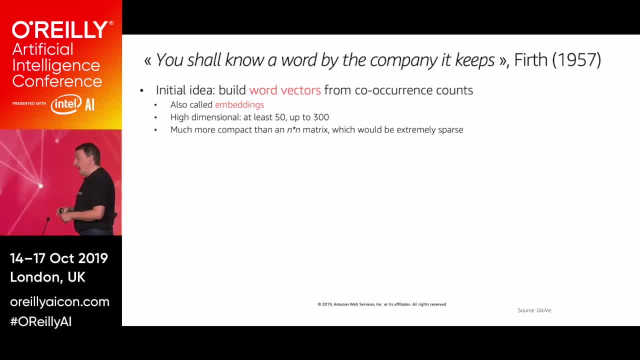 about context. Okay, Then you have to look, Okay, At words that are used close to this word. Okay, Because if a number of words are closely related, then of course, the probability of them appearing together is higher. And since we try to predict the next word, this is really the thing we're focusing on. 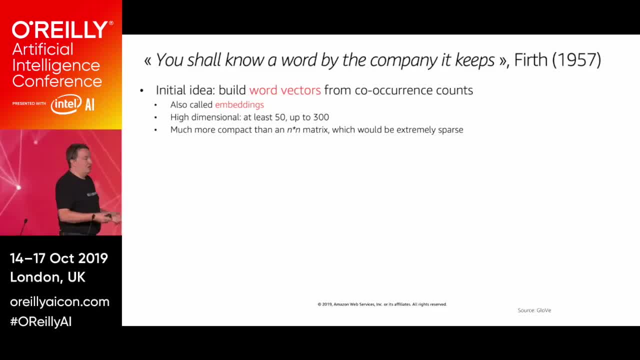 So the initial idea was co-occurrence counts. So just let's take a huge corpus, Let's build a big matrix showing how many times in a certain window So a certain pair of words will appear. And this is the starting point. The problem is: 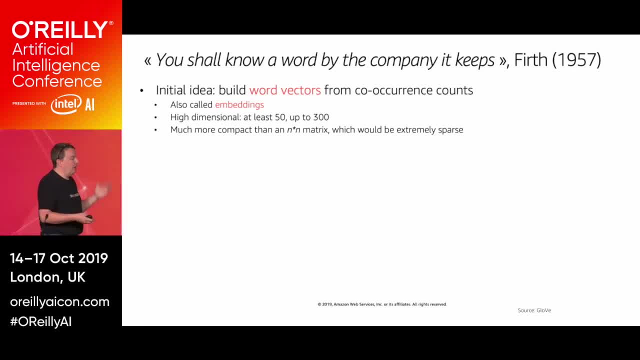 this is huge, Right? If you have a million words, then you don't want to be handling a million by a million matrix. So we need something denser, And this is the idea for word vectors: building denser, more compact representations of those counts. Okay, So 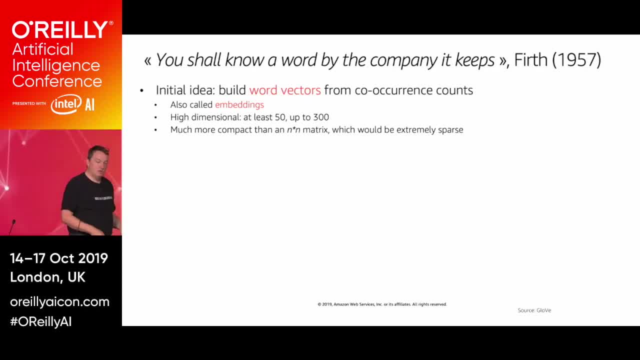 they're called word vectors. They're also called embeddings, because machine learning is a way to use very complex words for pretty simple things. I guess it's the curse of IT in general. They will have a couple hundred dimensions, So I guess from 50 to 300 is what we see, And they help us manage those relationships. 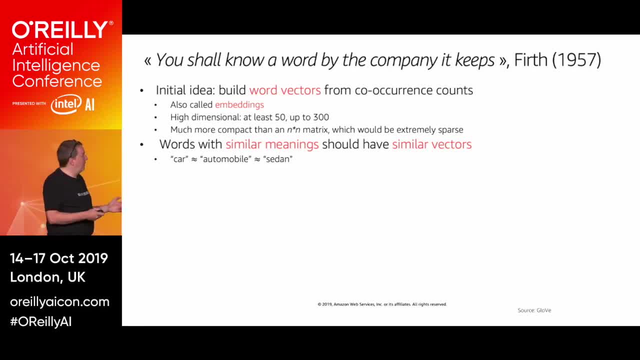 those counts, co-occurrence counts. The goal for those is that words with similar meaning, similar context, should have similar vectors. So the vector for car and automobile and sedan should be similar. They should be close, Okay, And we'll see what that means in a minute. And the distance. 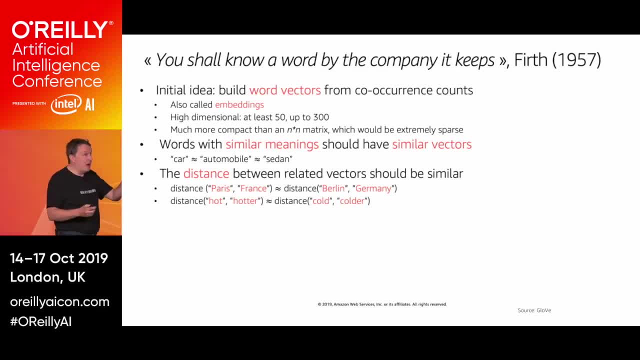 between related vectors should be similar. So the distance between the Paris vector and the France vector should be similar to the distance between the Berlin and Germany and hopefully London, UK et cetera. vectors Okay, And hot, hotter, cold, colder, Because 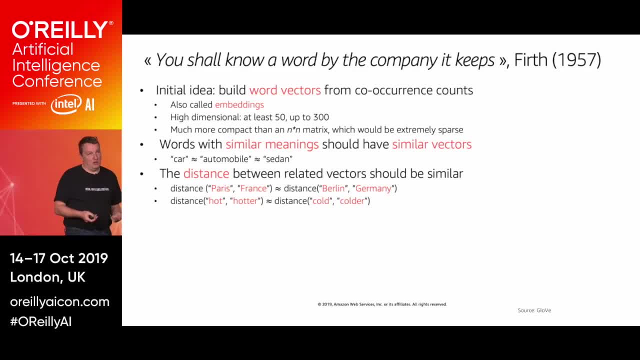 if, again, if those words are used in similar contexts, if those word pairs illustrate the same concept, then these should be reflected in their vectors. Okay, And these are some examples. So you know the vector between man and woman, from man to woman, the distance: 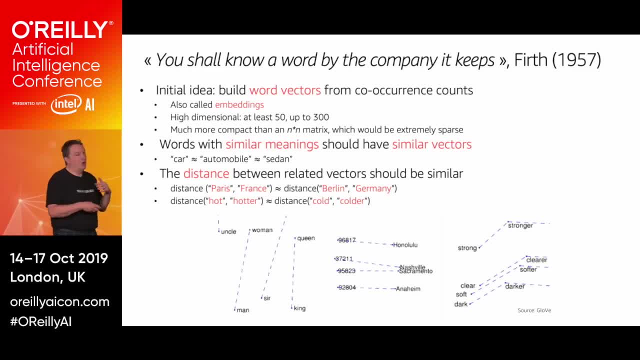 is kind of similar to king and queen and you know, hopefully other word pairs that reflect the man or male-female relationship. You know, same for zip codes, same for adjectives et cetera. That's the kind of thing we're trying to build And we'll see why that's. 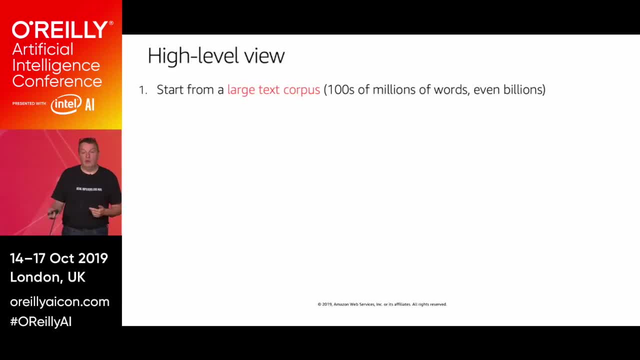 important. So the high-level view is: start from a mountain of data, Pre-process it. You will not escape data cleaning and data processing. So tokenizing, splitting words and punctuation signs, separating them with spaces, inserting beginning of sentence, end of sentence, et cetera, There's a whole 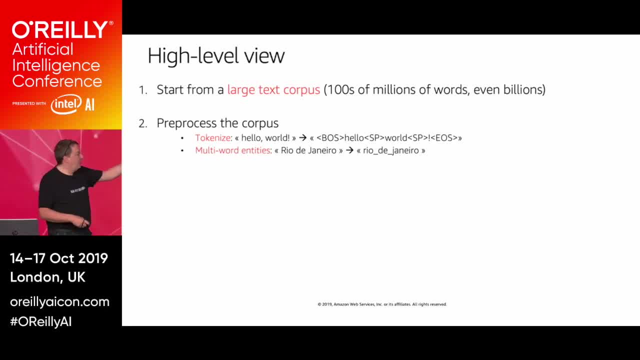 bunch of techniques. Maybe deal with multi-word entities. So I'm sure there's debate on whether this is a good idea or not. But okay, we could try this. Say, Rio de Janeiro is not one word, It's three words, It's actually one word. et cetera, et cetera. So plenty of techniques. 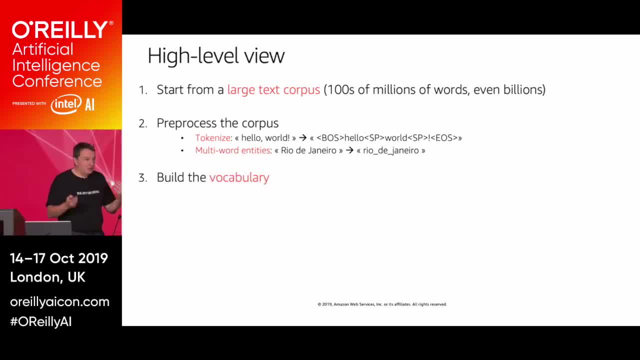 to prepare the data, Build the vocabulary. so the different, the collection of tokens, of different tokens, Learn vectors, Or maybe use existing vectors, or maybe fine-tune existing vectors. Okay, Because you can imagine some of that stuff is quite intensive and maybe 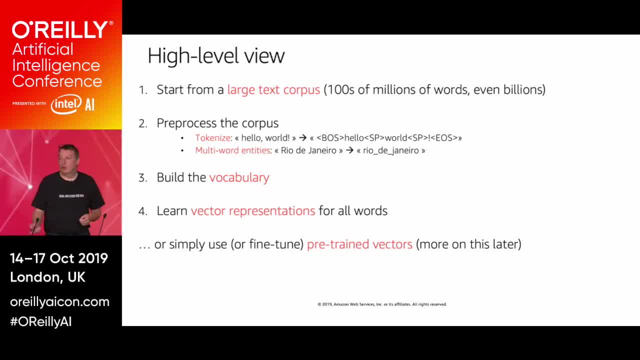 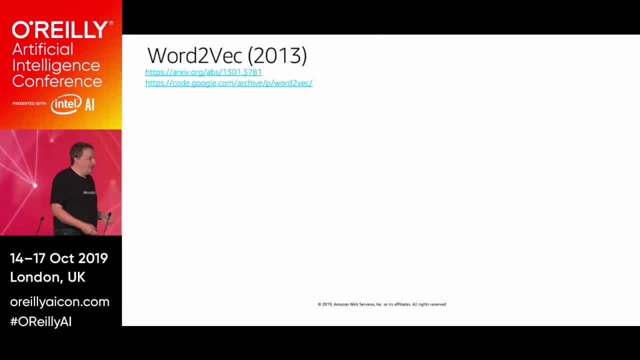 we want to spare the effort and the cost, So let's look at some algos, and of course, I'll use chronological order. So I guess the granddaddy, even if it's not that old, is Word2vec 2013.. And Word2vec is actually two different things. okay, Two different. 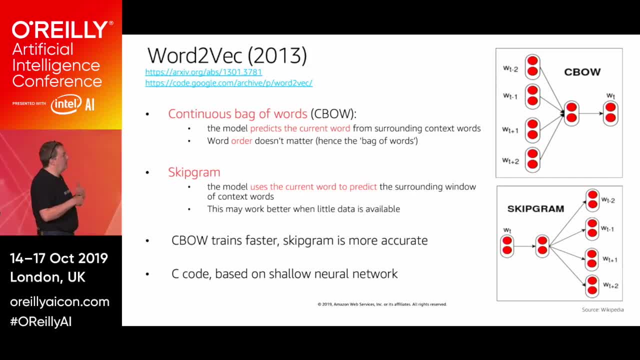 ways of computing and actually trying to predict the next word. So one mode is called the continuous bag of words. The bag of words thing means we don't care about order. Okay, So these are named the bag of words And we call it a bag of words model. In fact, we don't care. 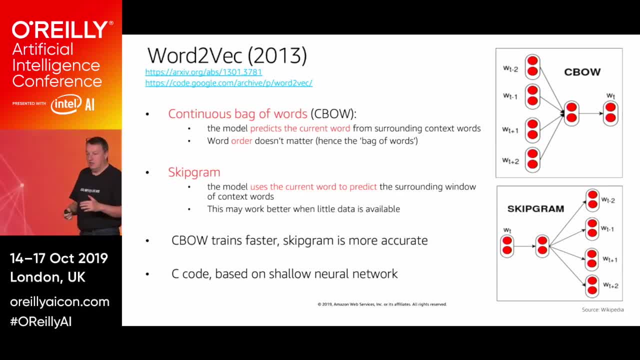 about order? We don't care about order. It's like the basic thing about the words model. The order of words doesn't matter And, as you can see, we use the surrounding words to try to predict the actual words. So an example would be this afternoon. 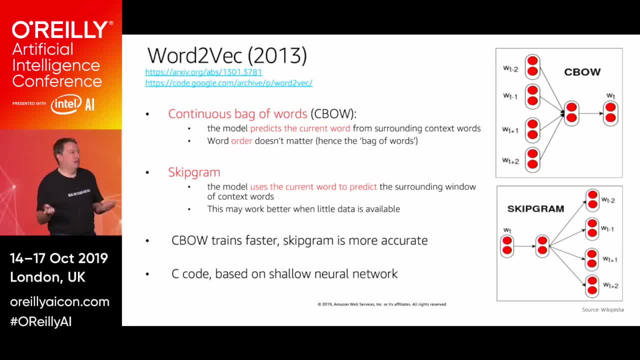 I will take the to Paris, France. right, And the best answer here would be train. okay, So you use neighboring words to predict the next. But order doesn't matter. okay, The skip gram mode is the reverse: You use a word to predict its neighbors. 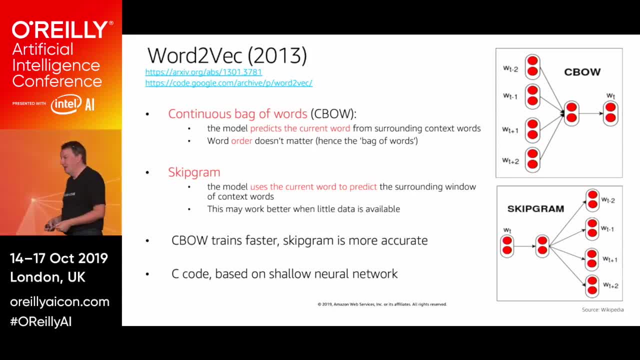 So I'll tell you train and you need to predict. tonight I'm taking the to Paris, France, okay, Which feels like a more difficult thing. but you can try both. One will generally work better than the other, okay. 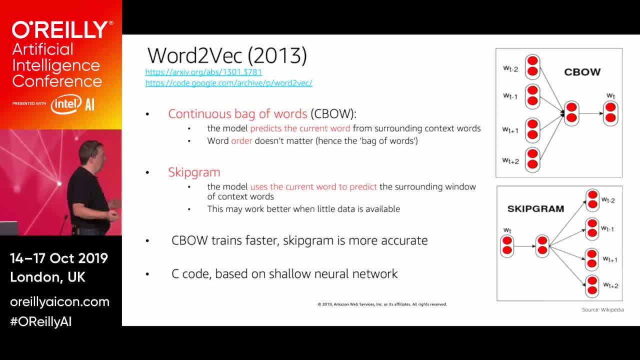 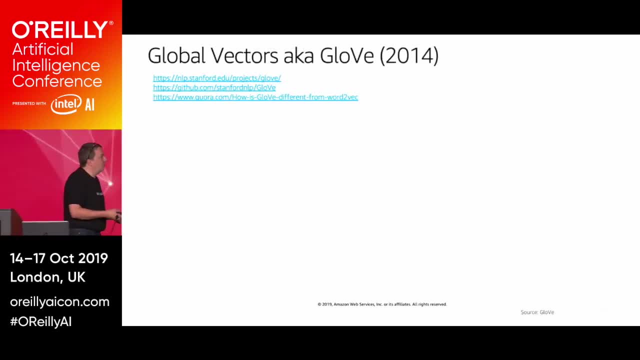 And this is C code. You can download it, compile it, run it. It's based on shallow neural networks. Shortly after that, GloVe came out. So GloVe is from Stanford University- And, of course, the research paper. well, 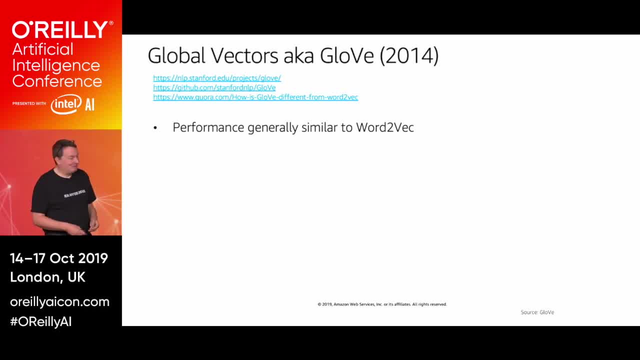 you know is making a point that GloVe is much better than Word2vec. okay, as you would expect, But now that the dust has settled on those- and I really read quite a few papers on that and read expert advice here and there- I think 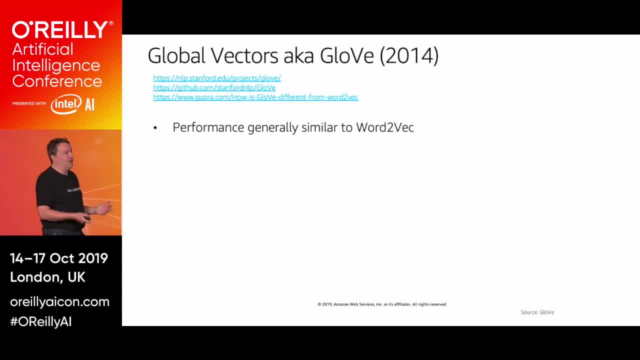 I think people generally agree now that you can get the same thing done. okay. If you use hyperparameter tuning specifically, you will get the same similar results. okay. So in some niche cases maybe one performs better than the other. but again, don't spend too much time. 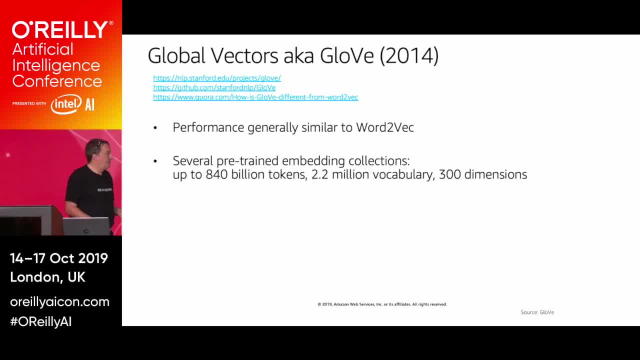 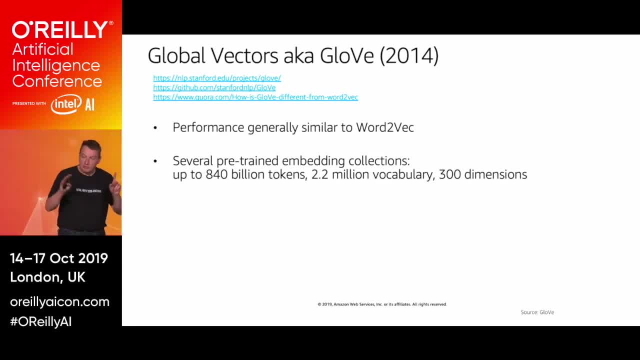 let's see, let's see, let's see. This is a collection of pre-trained embeddings, So you have small, smallish collections, but you have also really big ones, right, Like this one. I think this is the largest. 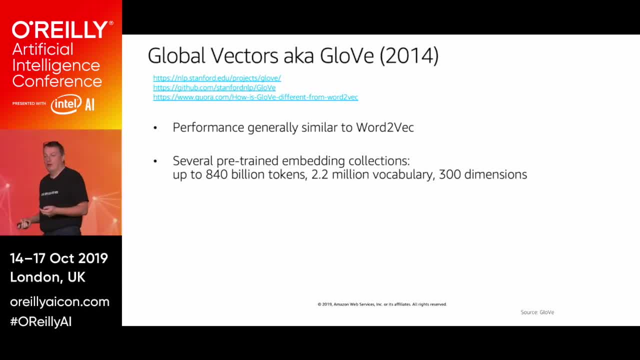 840 billion tokens, 2.2 million vocabulary, 300 dimensions. okay, And I believe this is in English, So that's a big one, right, That's a big one and it's a good starting point for your apps. 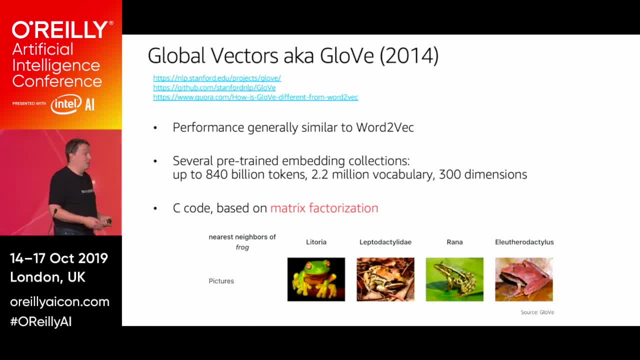 And this is C code and it's based on matrix factorization, which makes sense because, remember, what we're really building is this huge matrix. in this case, we would have a 2.2 by 2.2 million matrix with co-occurrence. 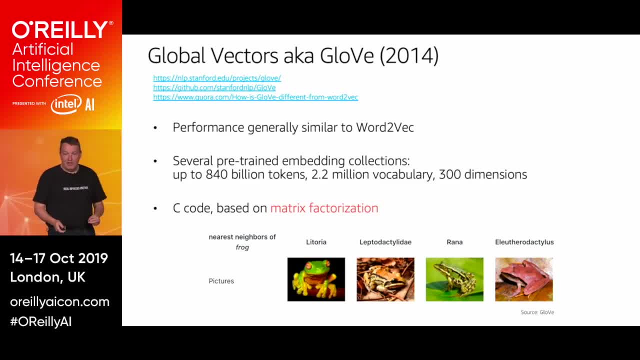 counts and we'll use matrix factorization to shrink it. okay, and so now this is an example from the research paper. actually, if you look for words that are closest to frog, this is what you get right. it's good they have pictures because, you know, for the life of me, i, i would never know. 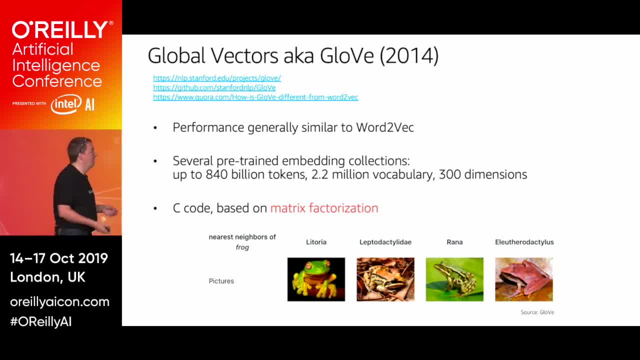 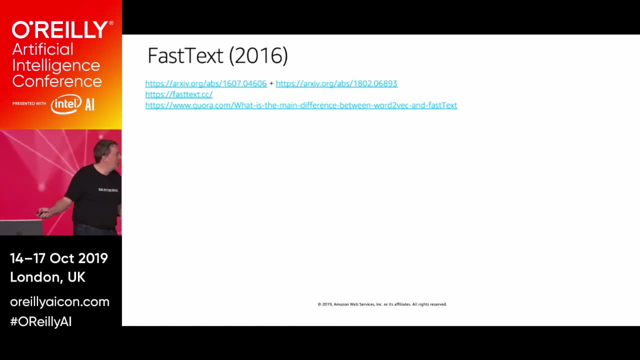 what a litoria, or leptodactyla, whatever is okay. so these are frogs, right, which i relate to for obvious reasons. okay, the next one is fast text. so this one is, uh, i guess, still heavily used. this was from from facebook, and what is it about? so it's an extension of word2vec. it's still doing. 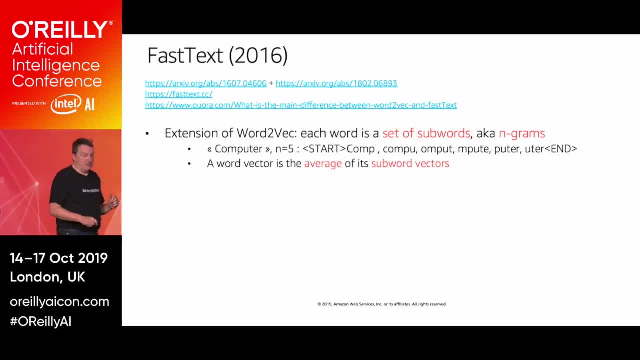 the same thing: computing, computing word vectors, but this time it's introducing a new concept called subwords. so instead of creating a vector for a word, it's actually looking at subwords, also called engrams, that make up that word. so, for example, if you use five character engrams for computer, 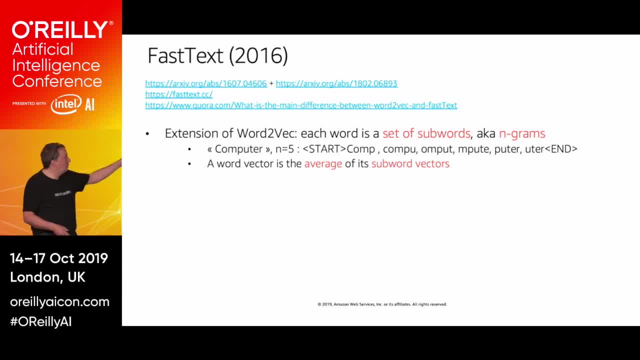 the engrams would be so: start of word, comp, compute, ompute, puter, uter, and a word okay, and you actually compute a vector, an embedding for each of those n-grams, And then the word vector. so the computer word vector is the average of those subword vectors. Again, this is a very confusing idea at. 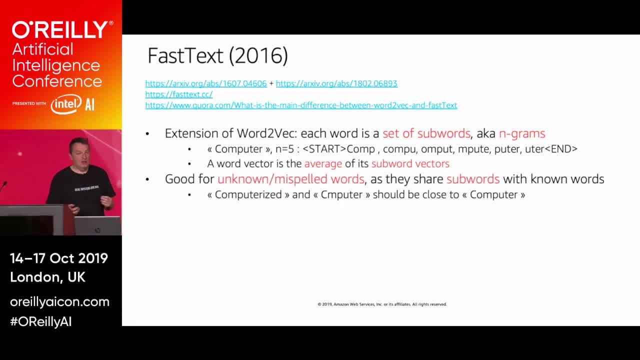 first, Why would we even do this? And the reason why we want to do this is because it lets us fix problems like unknown words, words that are out of vocabulary, right, If you try this with the other algos and you don't have a? 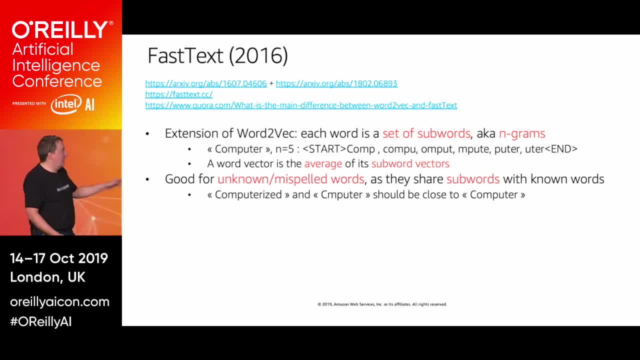 word in the vocabulary, then you don't have a vector for it. Now, even if you don't have a vector for computerized, which is a very weird word, or if you have a misspelled word like computer, then you can still. 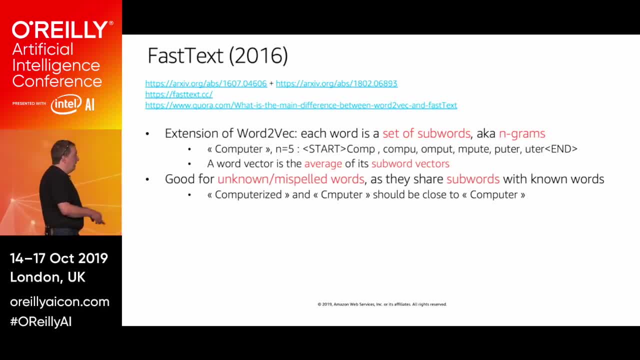 look at subword vectors and build a proper vector for each of those words And hopefully they should be close to computer because they obviously share subwords right, Make sense. So that's a big idea here And that's probably why FastX is very heavily used, So you can use it in. 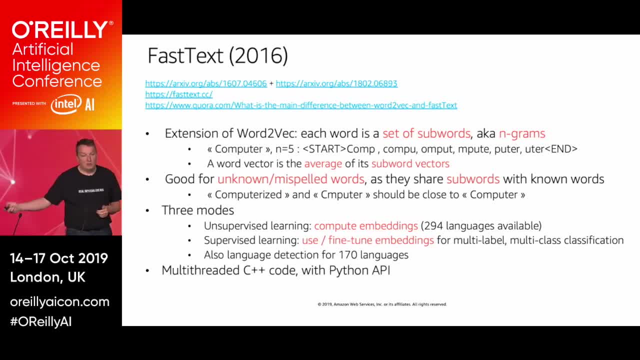 It's C++ code, it's super fast, hence the name Multi-threaded, et cetera. There's lots of good software engineering stuff in there as well, if you're interested, And you can use it in unsupervised learning mode. 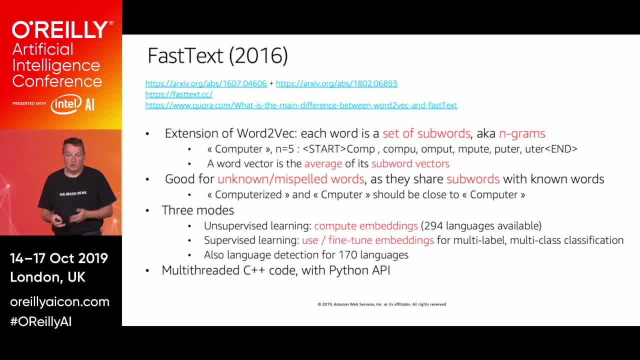 to compute vectors. They'll provide vectors for 294 languages, which seems like a lot, so should be able to get started quickly. You can do supervised learning for multi-label, multi-class classification and you can use or fine-tune embeddings on your corpus. 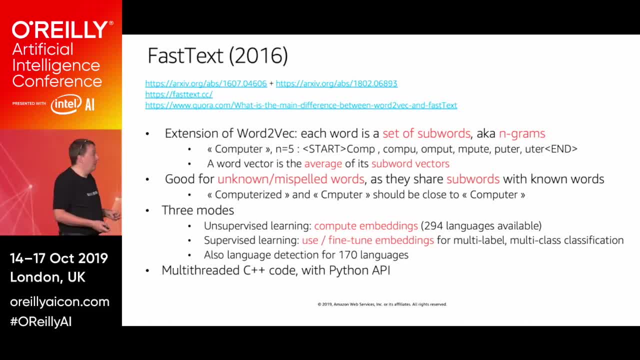 And it can also do language detection on quite a bunch of languages as well, So it's a really cool tool. Again, you can download it from their website, compile it. It's a tiny binary and you can run it in no time. 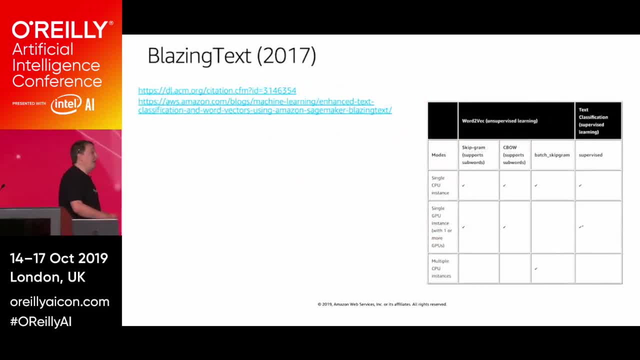 So that's FastText. So here comes Blazing Text. Of course there's a bit of competition, And this one is actually from Amazon. It was invented by Amazon, It was published, but the implementation, the code, is only available in our managed machine learning service. 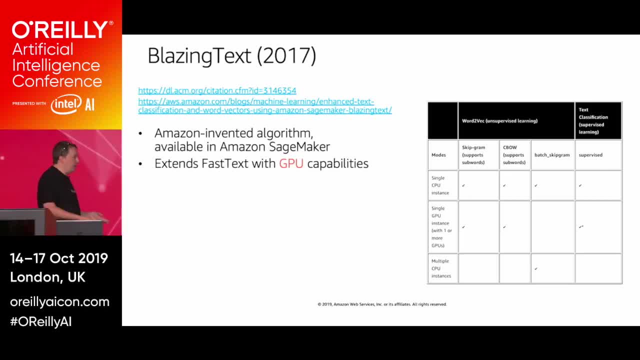 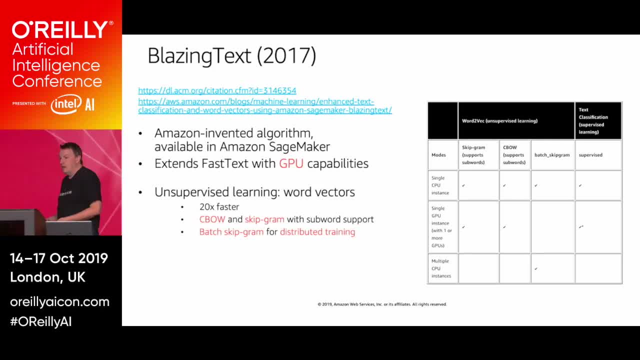 And now we can run Blazing Text, And now we can run Blazing Text On GPU, and so we can bring it to the next level of performance. We can use it in supervised learning mode- Unsupervised, sorry- And we find it's generally 20x faster. 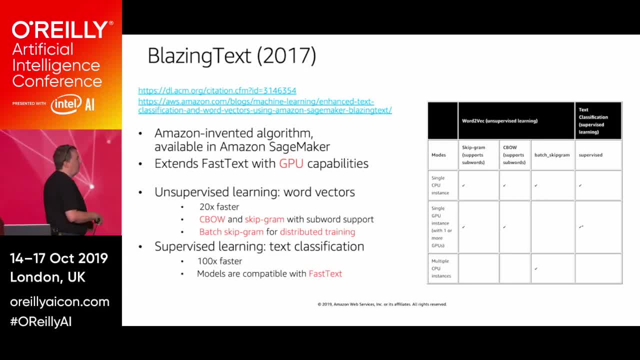 And we can use it in supervised learning mode and we find that it's about 100 times faster. So if you have small corpuses it doesn't really matter. I'll give you that If you're training on hundreds of billions of words. 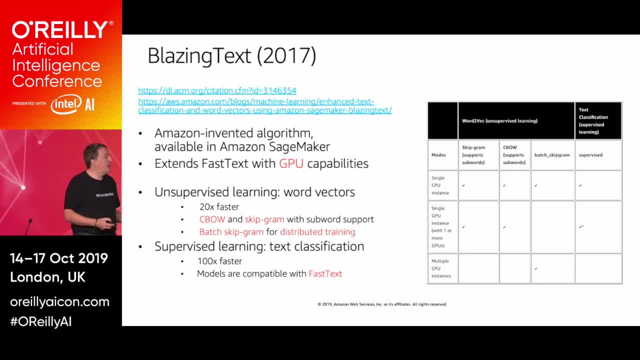 again, and again, and again and again. it's gonna make quite a big difference. And the cool thing is the models that you generate for so the vectors, and the model that you generate for classification is fully compatible with FastText, So you can grab the output from Blazing Text. 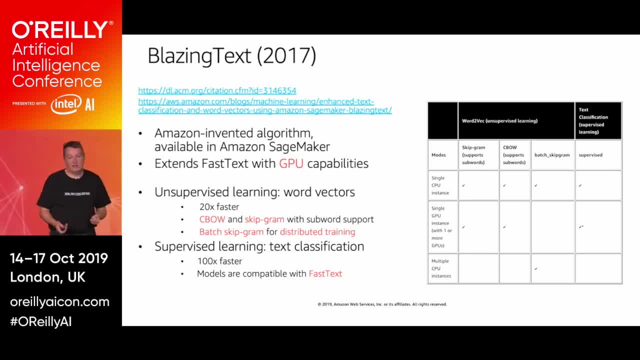 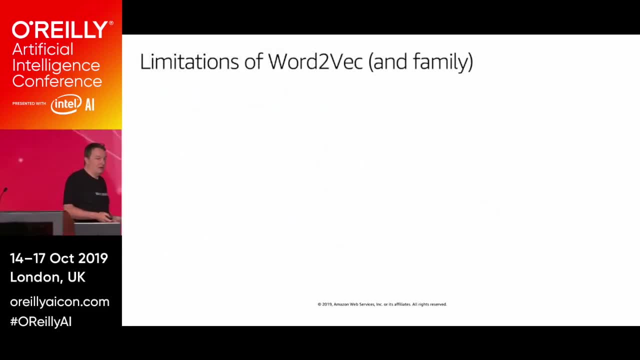 the binary file, load it with the FastText binary from Facebook and it works okay. So these are very nice, but of course they have some limitations. The obvious one is: what about polysemy? right, Kevin, stop throwing rules. 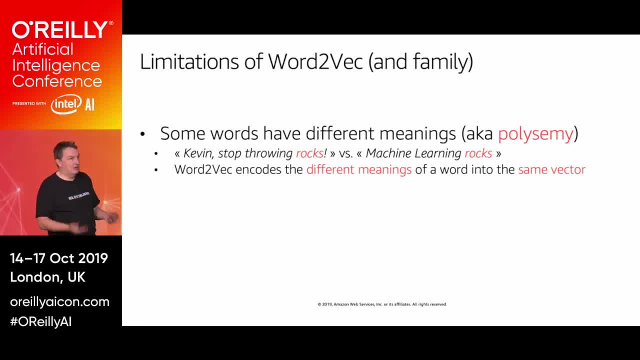 Okay, well, you have this code, and you have this code, and you have this code And you're gonna have a function called the machine learning rocks, because machine learning rocks versus machine learning rocks: Same word, same spelling, completely different meaning. 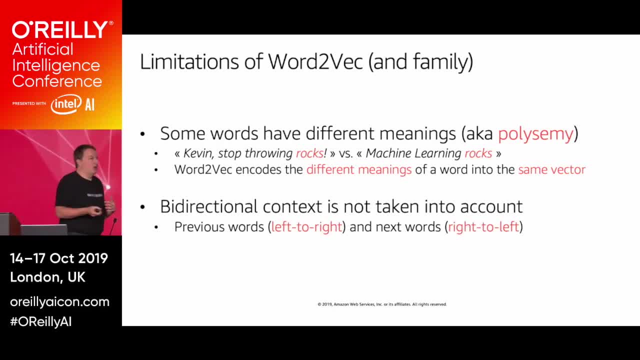 But with those algos you would still generate the same vector, right, Because you have one vector per word. The second problem is we don't really pay attention to bidirectional context. okay, We just look at the window right and we just count the words that are close. 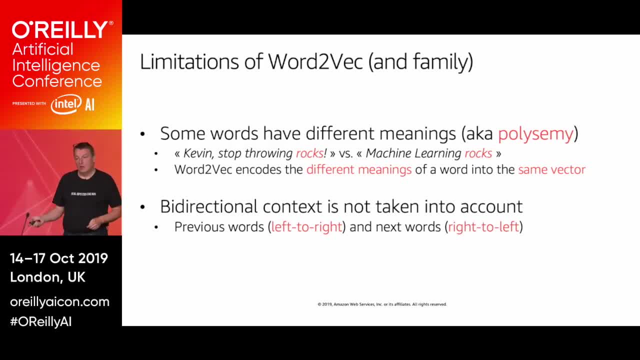 to the word we're interested in, but we're not paying attention to this, And so there was a big change at this point, right? So the word to vec and family are still extremely useful and well understood and easy to use, But starting last year, we had a whole new bunch. 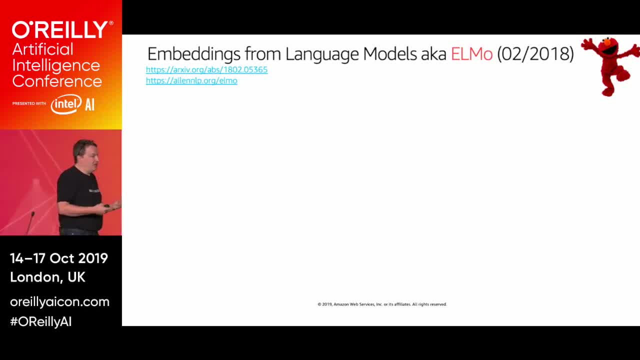 of algos showing up right And there seems to be a bit of a Sesame Street obsession here, which I'm not quite sure you know. I'm not sure what it's about, but it's there right, And hopefully you know what Sesame Street is. 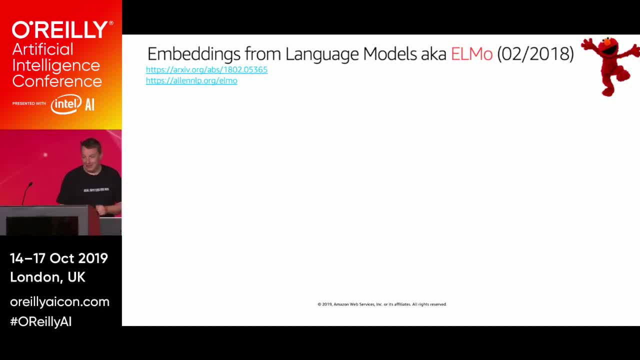 If not, then you were born too late, right, I guess. But you're young, so that kind of compensates for it. So Elmo. so the difference between Elmo and the other ones we're going to talk about is: now we're really 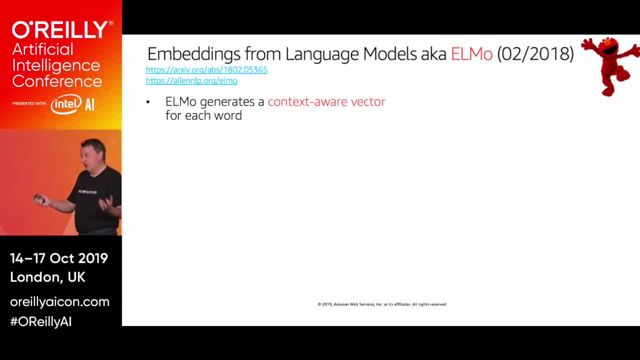 really looking at left to right, right to left, really looking at context in a finer way. So of course this means the architectures now become crazy complex. Whereas word to vec was a shallow neural network, GloVe was matrix factorization, et cetera. 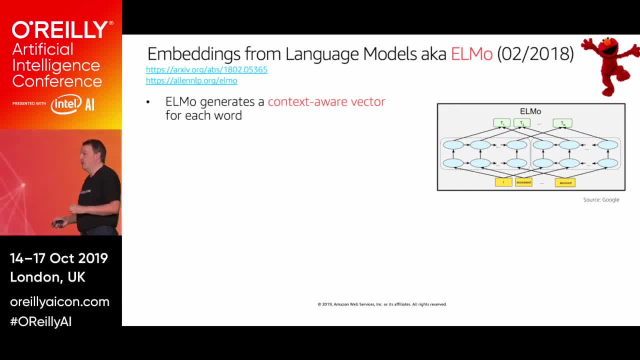 These go crazy on deep learning architecture, So it makes for very interesting reading when you read the research papers, but you're gonna scratch your head quite a few times and I am still scratching my head. So the first layer in Elmo is the character level. CNN right. 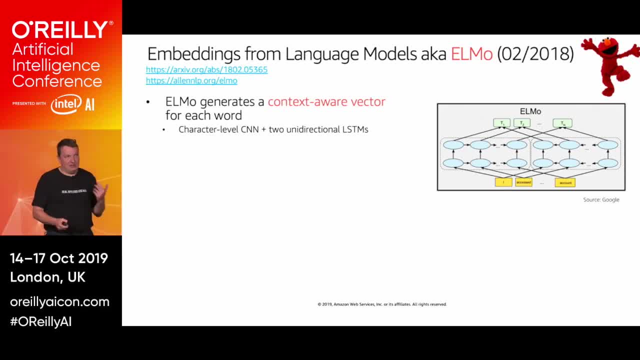 We know CNNs are great at picking up patterns, So I think it makes sense, from an intuitive perspective, that we start by looking for character patterns in the text we're trying to embed. Okay, and then it follows with two unidirectional LSTMs. 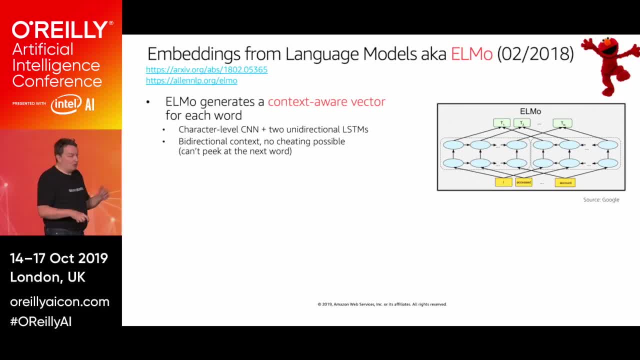 and the reason why you have to have one LSTM for left to right and one for right to left is because if you had only one right, Then you could cheat. okay, Because if we're trying to predict the next word and a single network sees the full sentence. 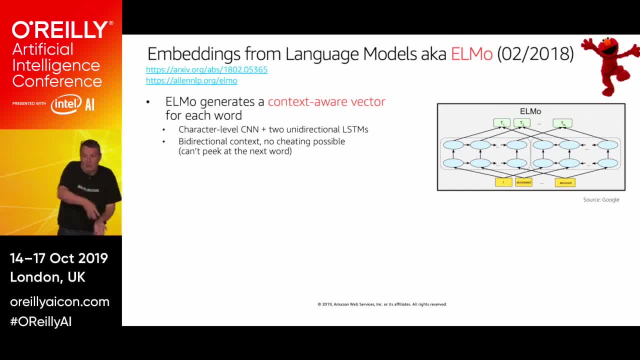 a single network could see what's left of the word and what's right of the word. So it's kind of cheating right? look at the future and as we have multiple layers, you could actually see the answer that you're trying to predict in the upper layers of the network. So that's not good. so to 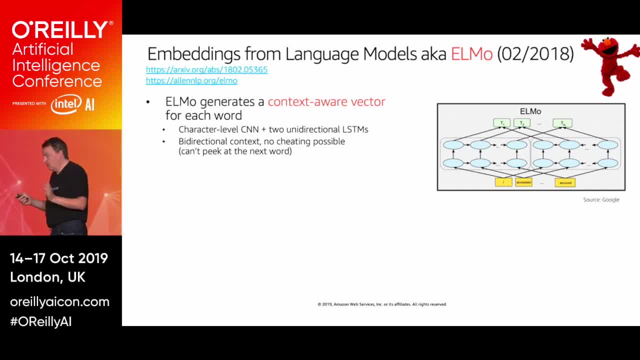 avoid that. they separate those two contexts- One is left to right, one is right to left- And the big change in ELMO is that the embedding that you get really reflects the output from those different layers. It's not just the output for the final layer it takes into. 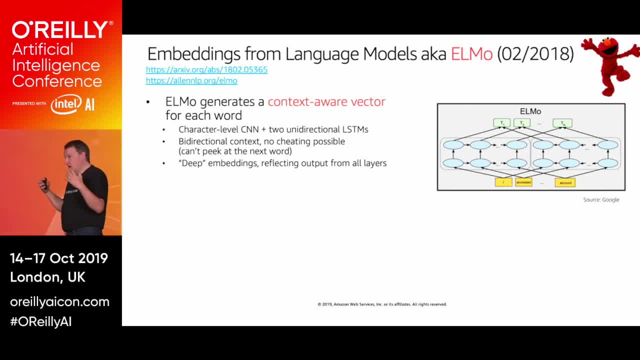 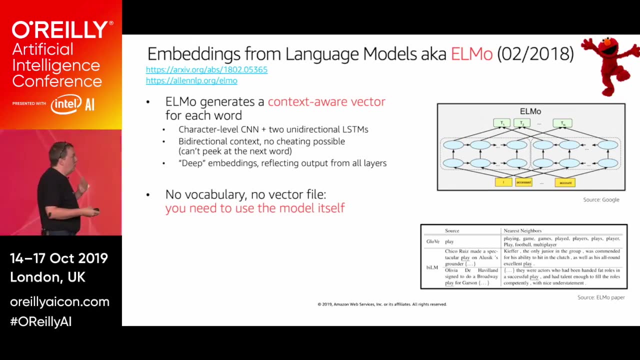 account, CNN context and context from both LSTM. So they refer to that as deep embeddings, because we see we learn stuff from all the layers. Another big difference is you are not generating a vector file. you are not generating embeddings just like we were doing. 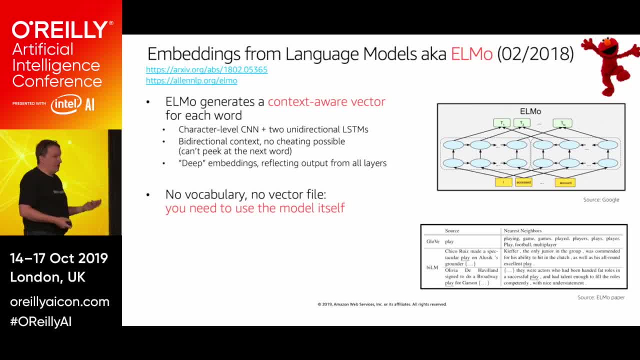 for the previous example, You need the model itself. The training process will learn the weights and all the parameters for the CNN and the LSTM. So you have to have the model to predict, And it's a good thing that they provide pre-trained models, because those things are pretty complicated to train. 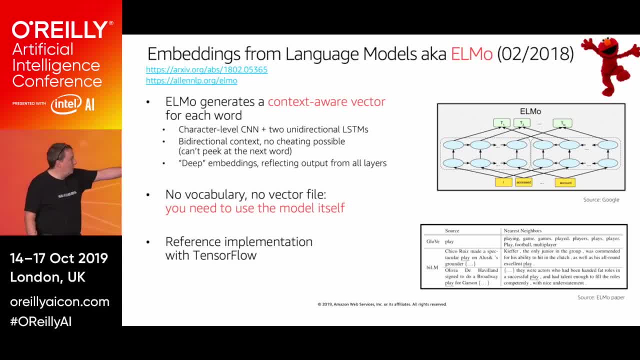 This is implemented in TensorFlow, by the way, so I'm sorry, it's probably a little small, but you can see in the top, sorry in the bottom, Sorry in the bottom right corner, the word play: so glove would have a single encoding. 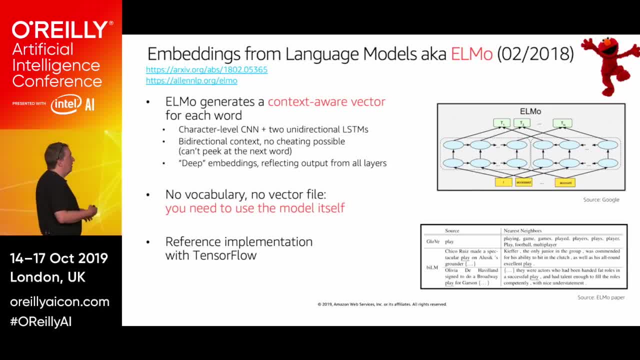 embedding for the word play. And if we looked at neighbors, similar vectors, close vectors, we'd find playing, games, played, plays, et cetera, which has a very heavy sports flavor to it. right? So that would tell us, hey, our corpus is using the word play mostly in. 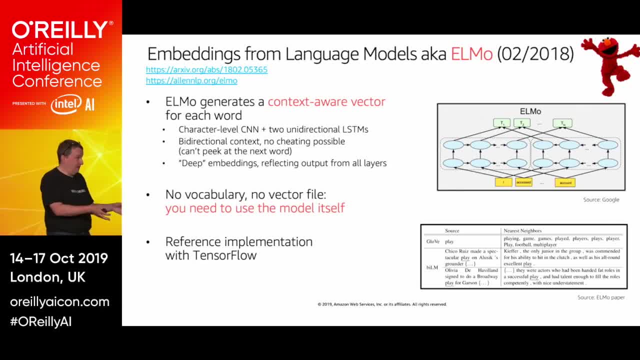 a sports context, And that's fine, right, That's the correct use of the word, But it's not the only use of that word. So now, if we look at Elmo, we can see two sentences here Chico Ru has made. 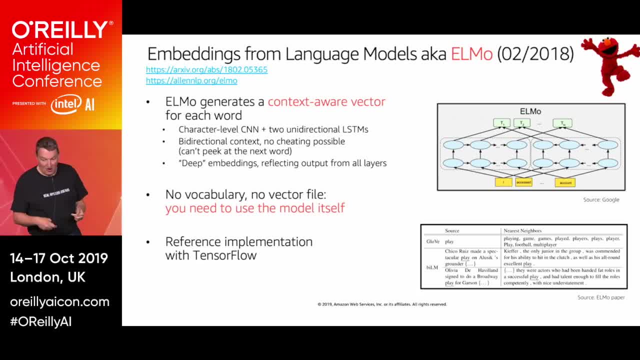 a spectacular play on a Lusix grounder, which is an obvious baseball reference, Or maybe it's cricket, Who knows right. And there's another sentence which is Olivia de Havilland's design to do a Broadway play for Garson, which of course is the same word play. 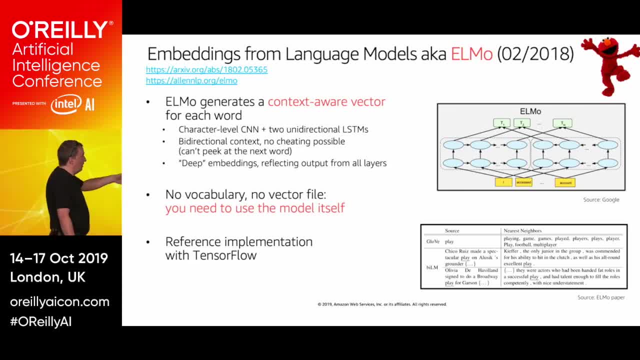 But once the first use is a sports context, the second use is a theater context. okay, And those are different. So now if we encode those words and we look for sentences in the corpus where we find similar embeddings, then the closest match for that first sentence would be kefir the. 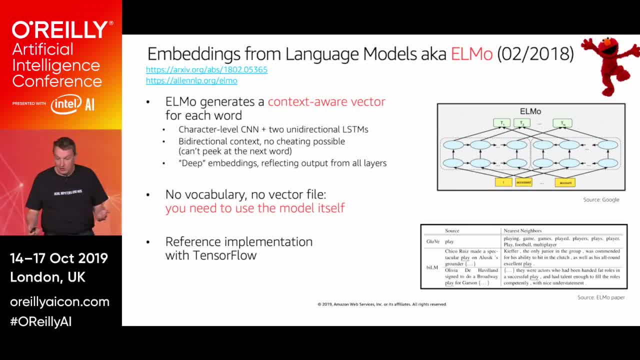 only junior in the group was commended for his ability to hit in the clutch as well as his all-round excellent play. So that means the closest use for the play word is sports. again And again. similarly, the closest use of the word play. 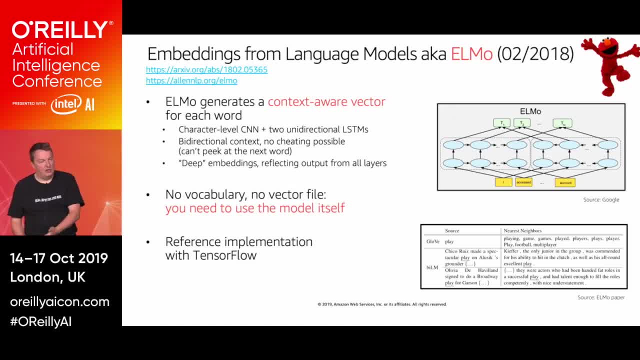 for the second context is another sentence on actors. So we see Elmo now is really taking context into account And it's able to generate on-demand embeddings based on what is actually around the word and not just looking at the word itself. This is a critical thing to understand. 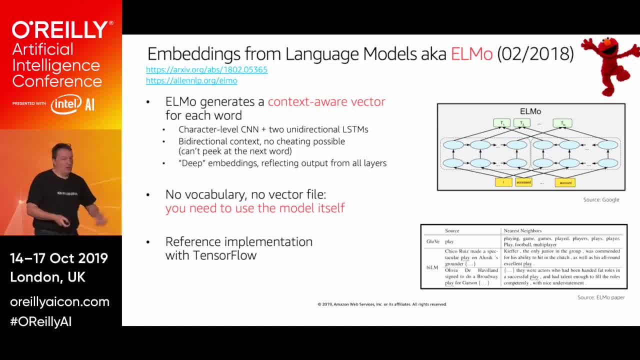 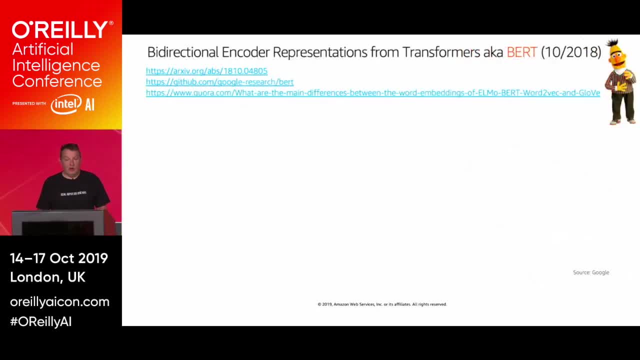 This is the huge difference between those new models and the older ones. Okay, make sense. And well, a few months later Bert showed up. okay, And Bert is just another of those interesting models, So it improves on Elmo in different ways. 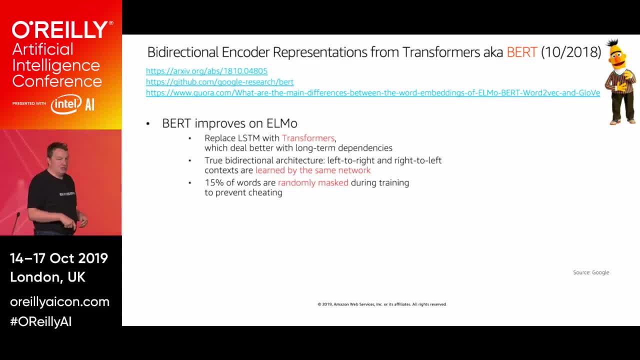 So the first way is it does away with LSTMs and it uses an architecture called Transformers, And the reason for this is basically Transformers are better at picking up dependencies than LSTMs. okay, So I wish I had time to talk about the Transformer architecture. 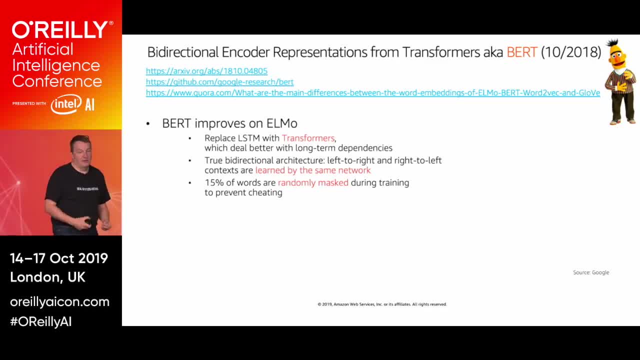 It's fascinating, It's based on auto-encoding, et cetera, et cetera. It's very cool stuff, but not today. So you'll have to believe me, they just do a better job. So Bert also goes with a single architecture. 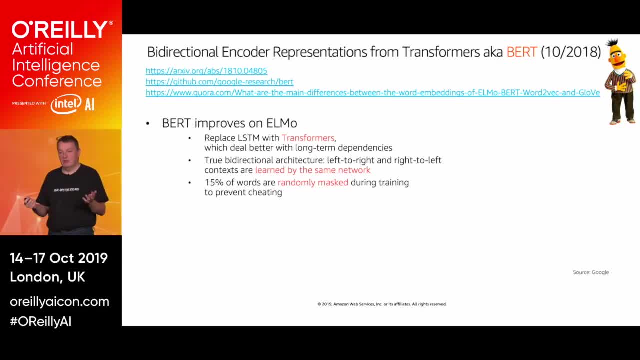 a single layer for left to right and right to left. okay, But what did I say before? I said: well, there's the risk of cheating if you will, if you don't know how to do that. There's the risk of cheating if you do that right. 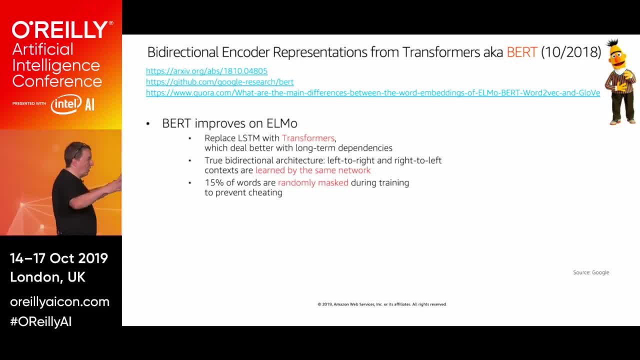 Because you feed the full sentence with the full context to a single layer, So it's gonna easily figure out what's the next word. So to prevent that, they use a masked learning where 15% of input words are randomly masked, So they just replace 15% of the words randomly. 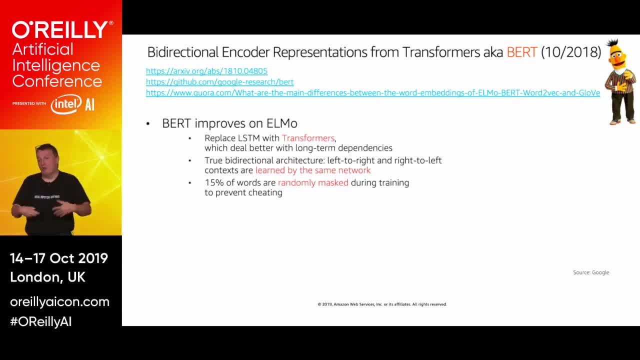 with a token that says mask. So they throw a wrench into the learning process. That's the training process, so to speak, And it looks like it's enough to prevent cheating. okay, So again, pretty complex architecture, but the difference with ELMO is single layer. 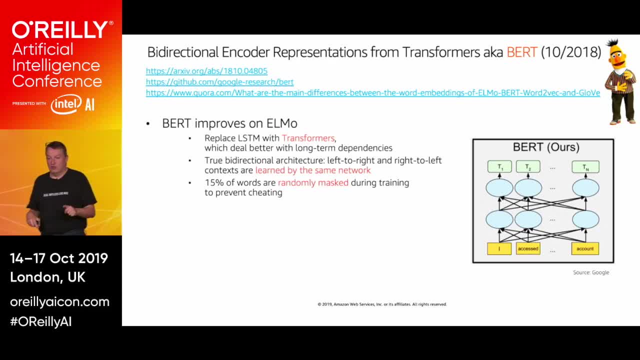 or single network for both contexts, And we fix the cheating problem by randomly masking words during training. You get two pre-trained networks, So Bert Bayes and Bert Lange. Okay, Lange is pretty large, So if you're downloading them you might wait a while. 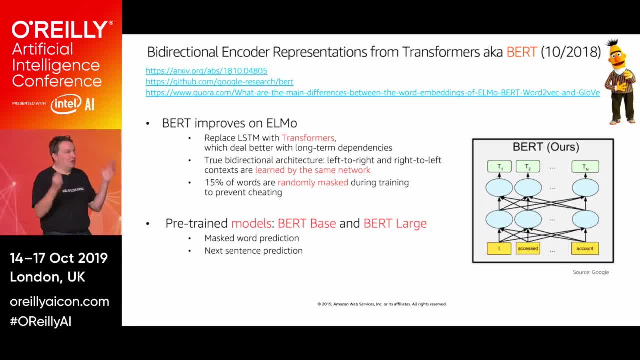 And these are trained on mask word prediction. Okay, so giving a sentence with mask words and figuring out what are the mask words, And it can also predict the next sentence. So here's the sentence predicts the next one. Okay, and these also come with. 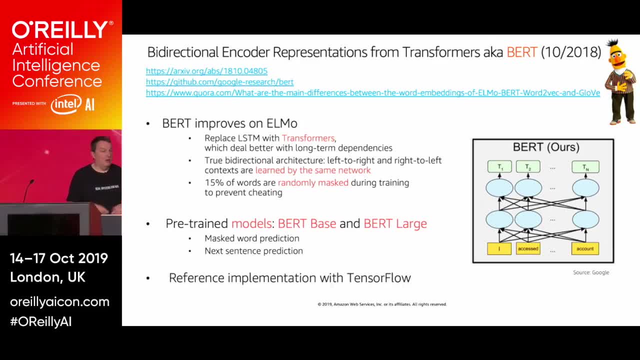 if you look at the GitHub repo, you'll find scripts, Fine tuning scripts, et cetera. Unfortunately, no notebooks. So my initial reaction to this was: wow, this is gonna be a headache to use. And yeah, it's a bit of a headache to use. 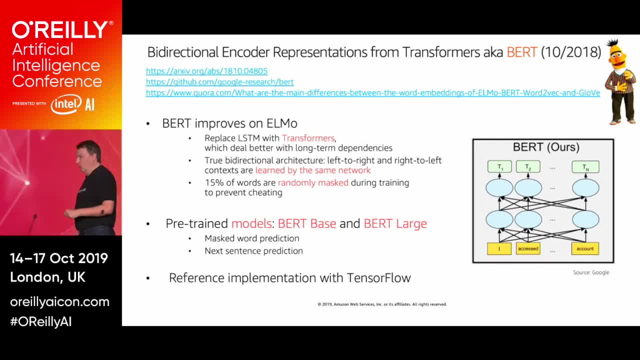 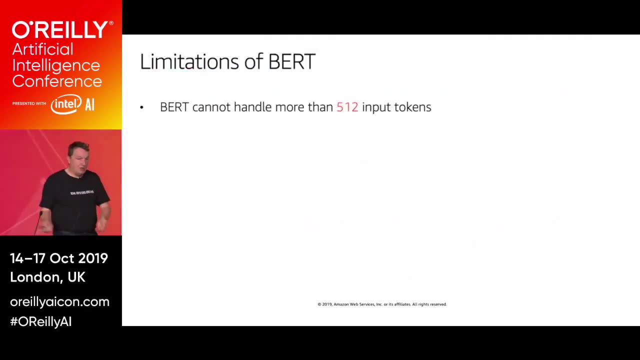 I think this is not super intuitive- all those scripts- But okay, you'll figure it out. And there are plenty of good blog articles that show you how to do this. So here's Bert. And again, Bert has limitations Right now. it can only handle five. 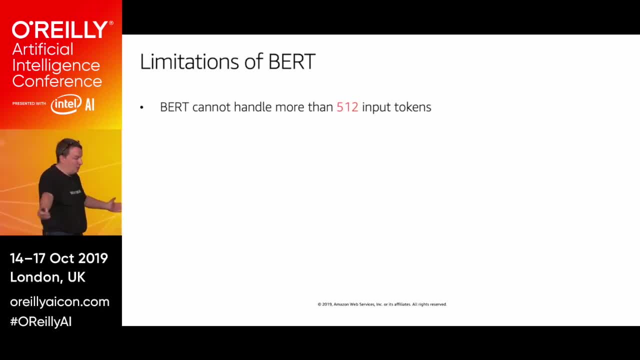 hundred and twelve input tokens, So you can't really learn super, super long bits of text in one go. It does mask words during training, But if you fine tune, you fine tune with the full text. So this creates discrepancy between training and fine tuning. 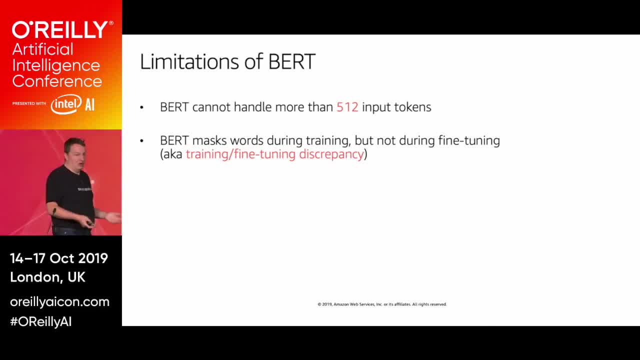 And it's not entirely clear how Bert resolves that thing. Okay, so there's still discussion on is this a major problem or not, And is the algo actually taking it into account or ignoring it? But you might see some different results here. 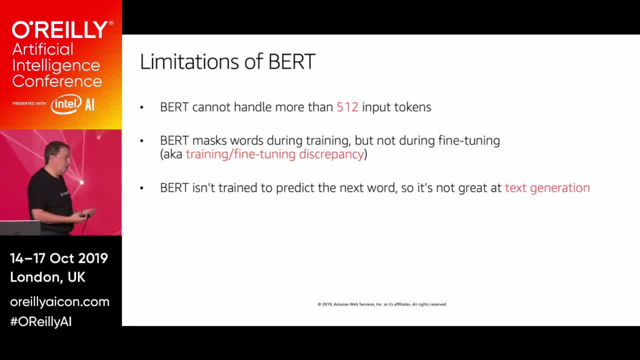 So, Bert, or at least those pre-trained versions- they're not trained to predict the next word. So text generation is not one of the tasks that Bert is great at, if you use those trained networks. And of course, he doesn't learn dependencies for masked words. 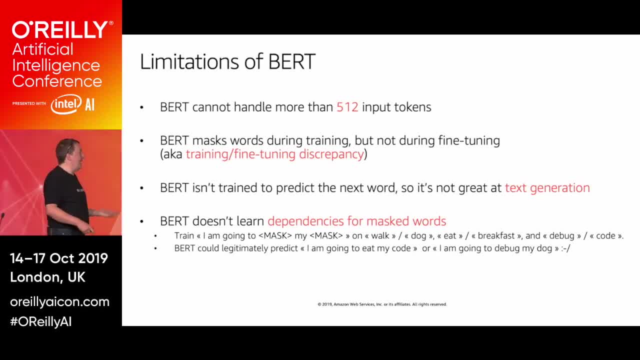 So if you train it on- I'm going to mask my mask right- And your corpus said: I'm gonna walk, I'm gonna walk my dog, I'm gonna eat my breakfast, I'm going to debug my code, Then of course it could legitimately predict: 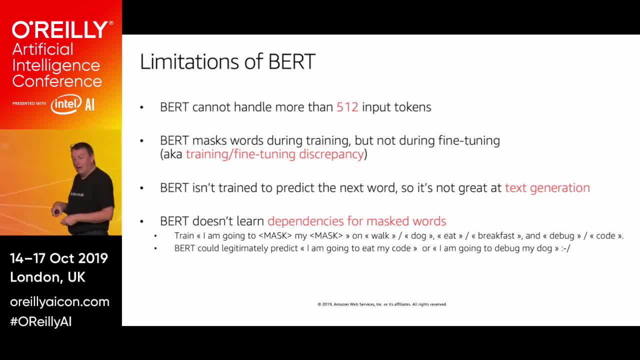 that I'm going to eat my code or debug my dog and things like that. So that's the issue you get with masking. Sometimes it may just completely miss the target. So the sentence will actually be correct, maybe grammatically, but from a meaning point of view. 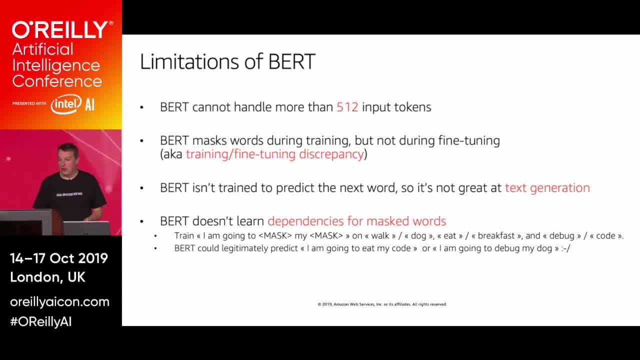 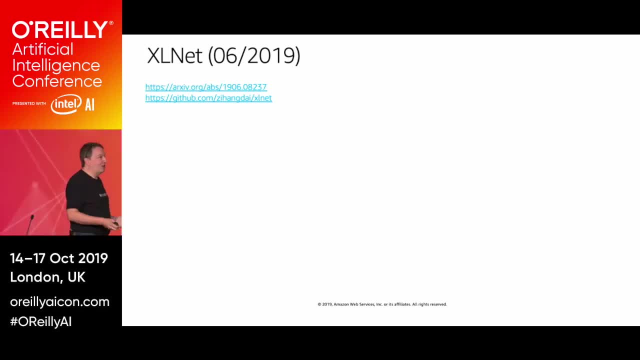 it's gonna be completely wrong. Okay, still, I mean, this is a great advance And it goes on. Okay, ExcelNet. So I guess they couldn't find an acronym for a Sesame Street character, or they didn't think about it enough. 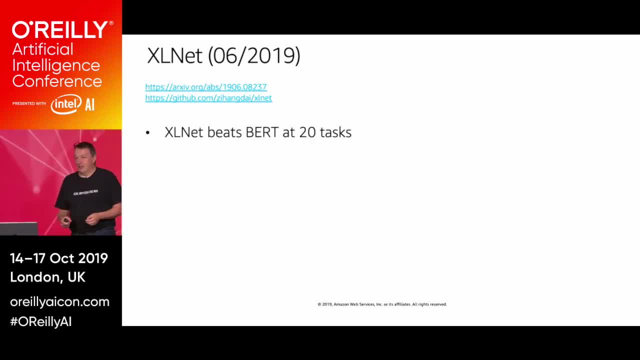 Or maybe they just didn't like Sesame Street. And ExcelNet was released this summer and it improves on Bert at 20 tasks. So, as you can guess, there's a bunch of benchmark tasks reflecting all those NLP problems we discussed. so sentiment analysis and next word, prediction. 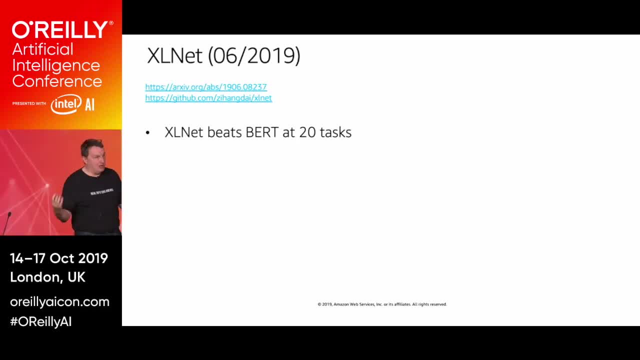 and sentence pair classification and translation. So a set of benchmark tasks that kind of represent NLP problems And this is how researchers measure the improvement on state of the art. So this is a significant improvement. ExcelNet uses bidirectional context as well. 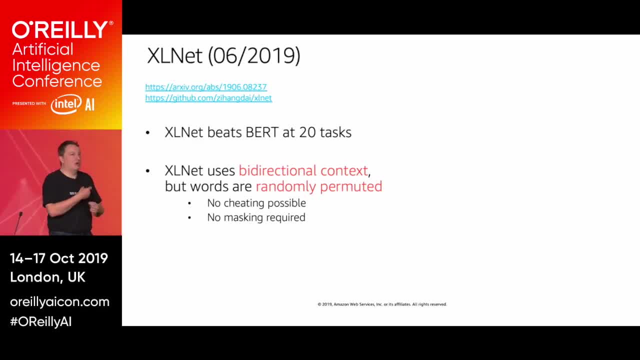 but it does away with the masking And it randomly it puts words right. So it's looking at neighboring words, but it does move them around and learn different combinations, okay, So no cheating, because you don't know if a word to the right. 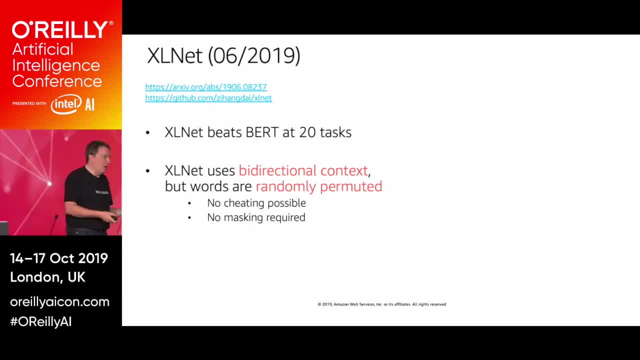 is actually. maybe it came from the left. So whatever expectation you had on that is broken, I guess, by the permutation, And it doesn't need masking Again. you get two reference models: ExcelNet-based, ExcelNet-large. 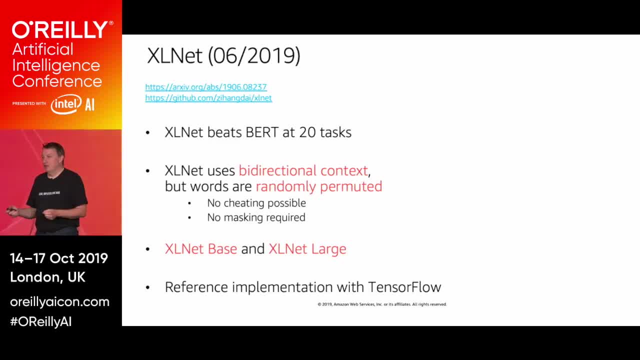 And these are pretty much the best today, except no, Yeah. So I started working on this deck this summer and it's a challenge, okay. And so in just a month later- which, by the way, shows you the acceleration that NLP is. 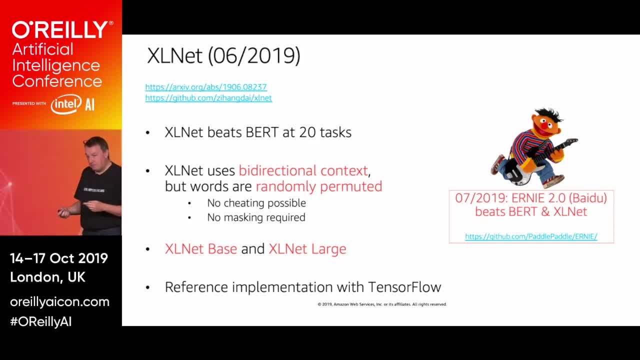 is experiencing today And I think that's, you know, that's not stopping anytime soon. I think that there are it's improvement after improvement, Just like we had that for computer vision, you know, maybe six, seven years ago. 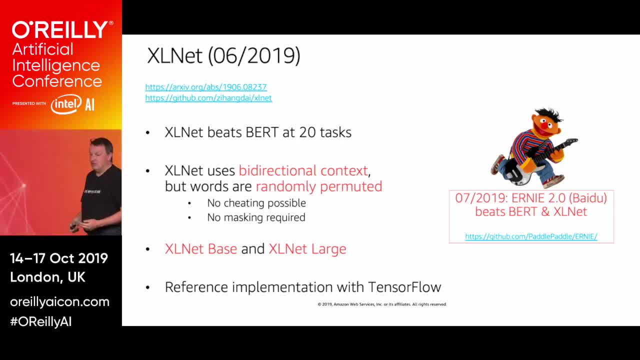 Every year you would have a. every month you would have a new CNN architecture, improving on ImageNet task, et cetera. I you know, I guess we see kind of the same thing for NLP now. So I'm thinking 2020 will be the year of NLP, but you know, 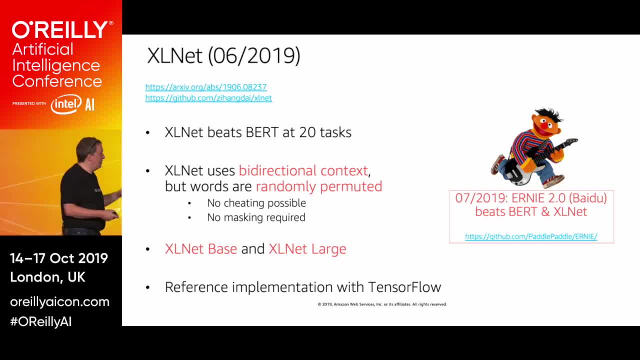 So I'm thinking 2020 will be the year of NLP, but you know. So I'm thinking 2020 will be the year of NLP, but you know, But maybe it's just me. So anyway, just a month later, 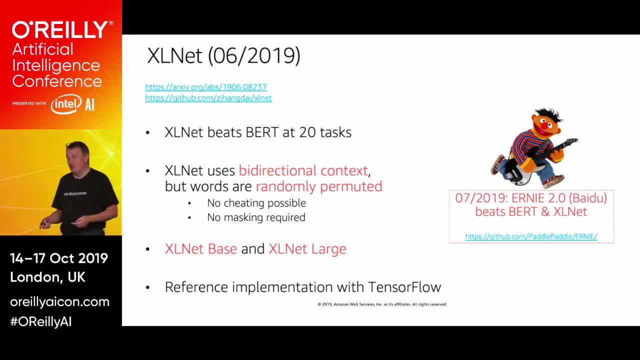 Baidu released Ernie, so Ernie 2.0, so the improved Ernie that improves again. on BERT and ExcelNet. Okay, And I think that's pretty much where things are right now And you know, of course they're still. 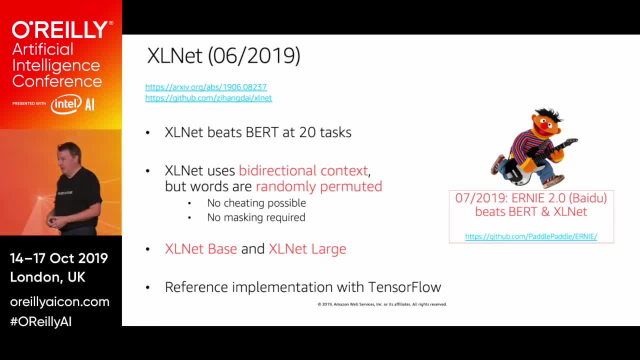 everyone's still competing on this And I'm sure we'll see some interesting models. But looks like this is pretty much what you know. But looks like this is pretty much what you know. But looks like this is pretty much what you know. 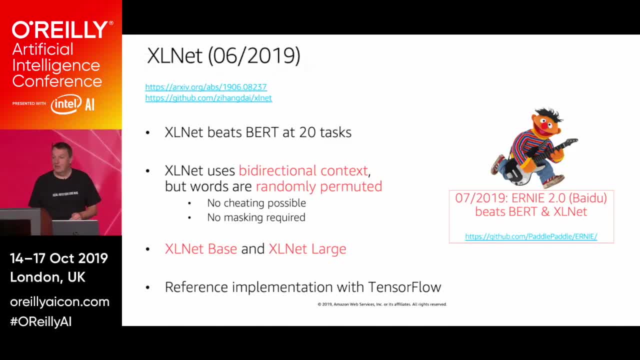 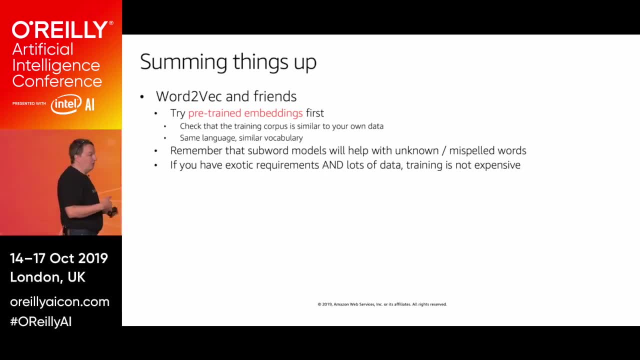 you know Ernie ruling the show at the moment. So, okay, it's all nice and fun, but what do we do with this? So, if you want to work with Word2Vec and friends, because you need embeddings, you don't want to carry. 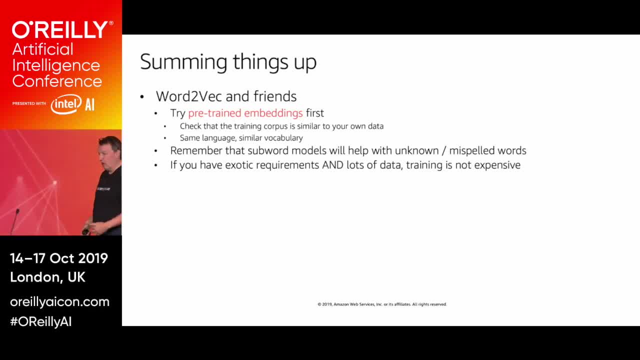 that big fat model with you and they feel too complicated. that's fine, They work still very well. They provide you with pre-trained embeddings. They might just work out of the box for you if you want to, if you use a general purpose English text. 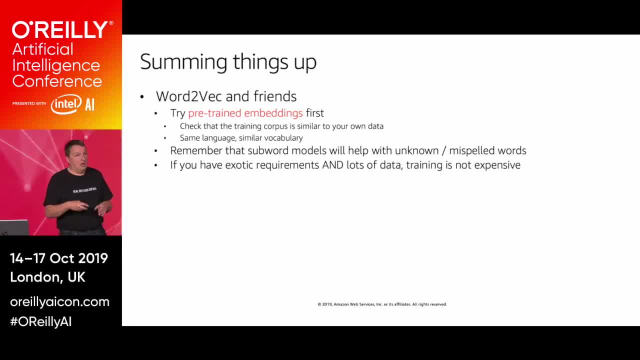 let's say it's going to be fine, Just make sure the corpus looks like your data. Obviously it needs to be in the same language and with a similar vocabulary so you can run some stats. but I would say generally, you're in good shape. 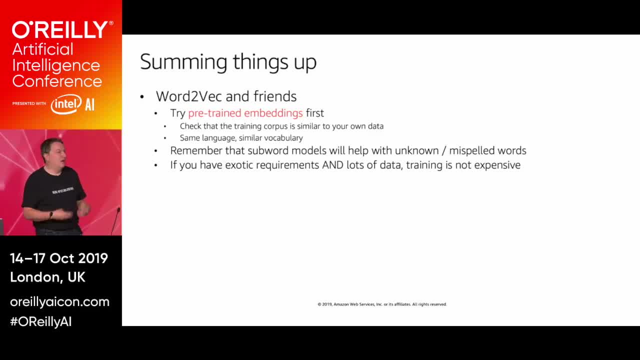 Subword models are really interesting. If you have misspelled words, unknown words, they're gonna help you out and they might actually save you from running spell checkers and all that stuff. So if you have exotic requirements, so if you're dealing with medical vocabulary, 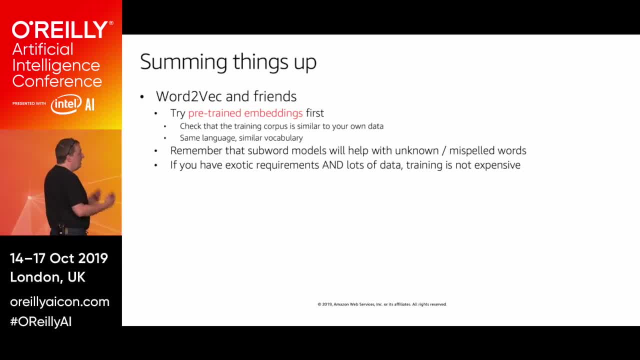 or legal vocabulary- I mean extremely niche words- then maybe it's worth training your own embeddings or fine tuning on your own corpus. if you have enough data, Training is not really expensive. for those All the new guys, training is super expensive, so don't try. 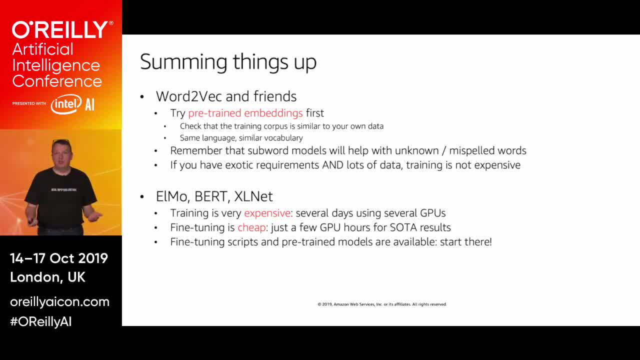 It's gonna take, it's gonna run for days on many GPUs and that's the reason why they do provide you with those pre-trained models. Fine tuning is quite cheap, so that's the better option and, like I said before, you'll find fine tuning scripts. 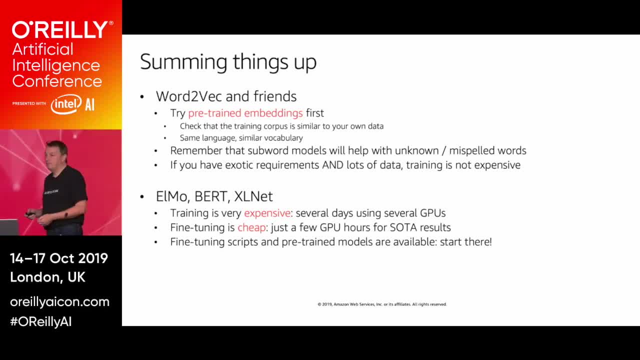 pre-trained models and you can start from there. okay, And never forget the best model. okay, because that's the question I get: What's the best model? So I don't know. the best model is the one that works best. 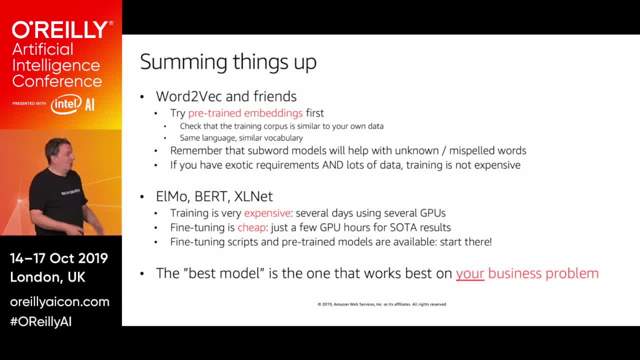 on your business problem, okay. So once again, don't avoid hype-driven development and hype-driven machine learning. Try different things. Maybe you find that fast text is more than enough. you know runs 100 times faster than everything else. 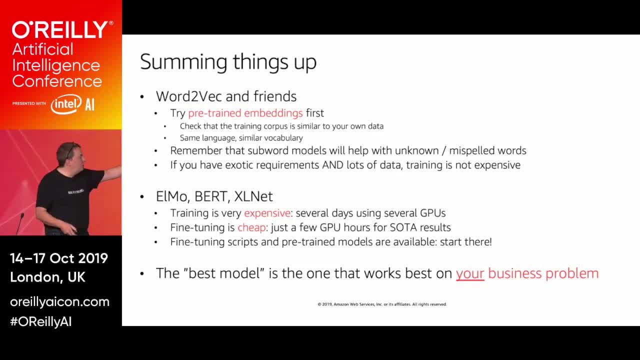 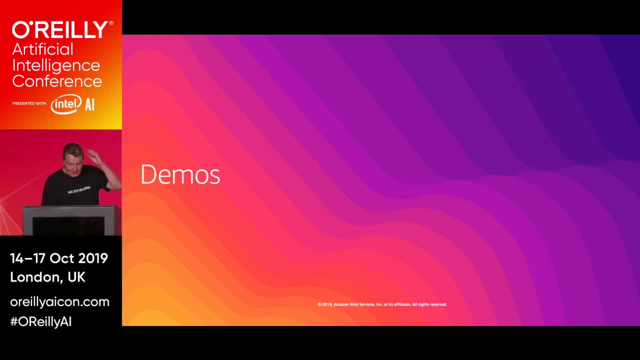 and that's the one you go with, okay? So don't rush to those new things just because they're new. I don't think it's good practice. So let's do a couple of demos. Really quick demo. Here we go. 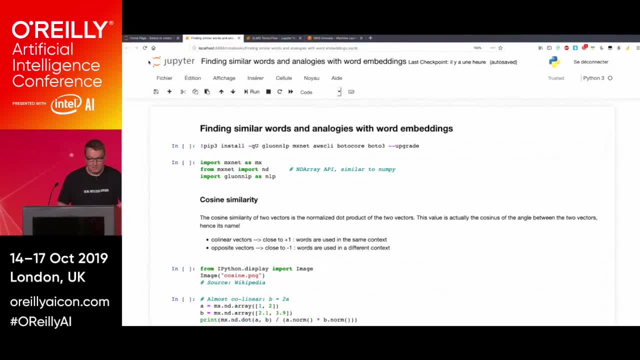 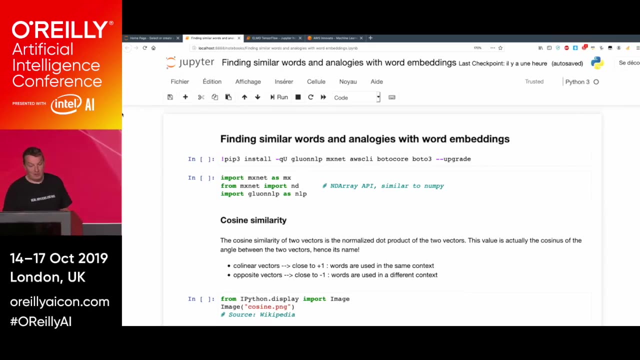 So the first thing I want to show you is how to use Word Vectors. Can you read okay in the back? Yes, Okay. I want to show you how to find similar words and analogies with Word Embeddings, So I'm gonna use MXNet and GlueOn and LP. 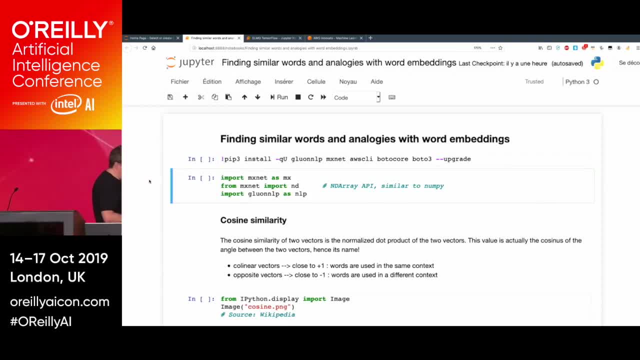 So GlueOn is an imperative API on top of MXNet and if you're interested, run that okay. and similar to PyTorch, let's say, And it has a bunch of toolkits and gluon-nlp is one of them. 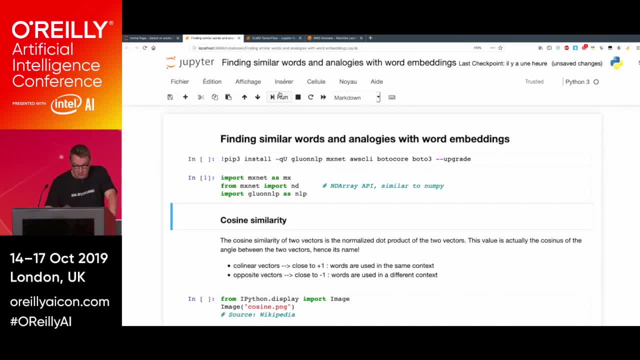 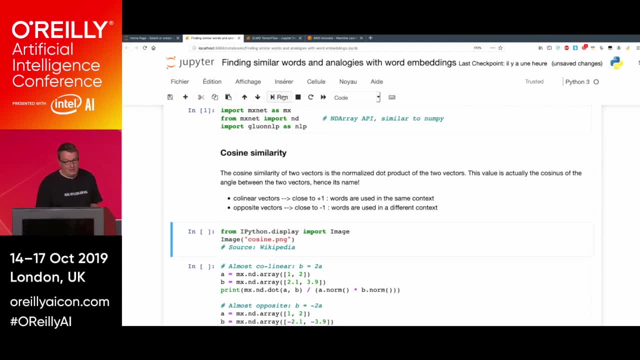 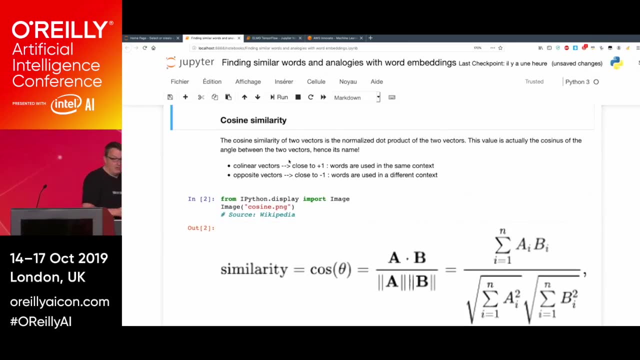 Okay, so let's import that stuff, And this is running locally on my machine, So hopefully it doesn't crash. So first we need to understand how to compare vectors, And we use this metric called cosine similarity, which is just a normalized dot product. 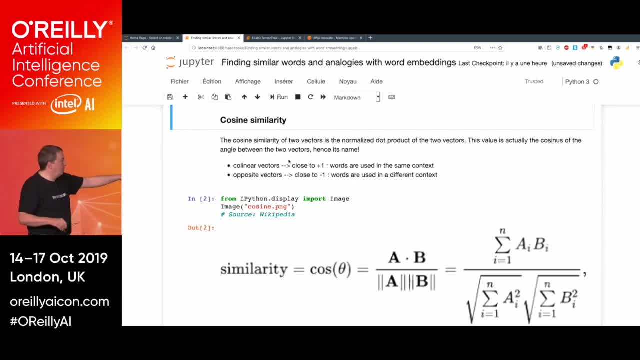 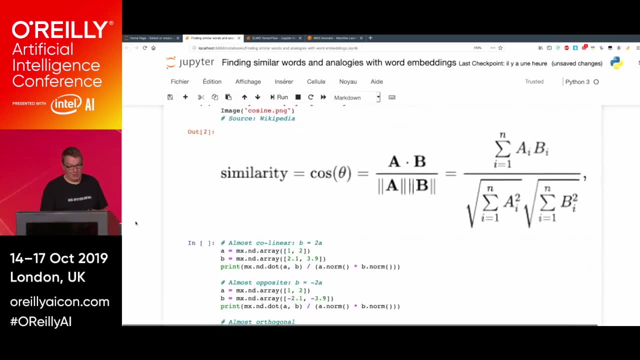 Okay, so we take two embeddings, two vectors, compute this: If words are close, then vectors are close, then the cosine similarity is close to one. If the words are opposite, then the vector cosine similarity will be close to minus one. 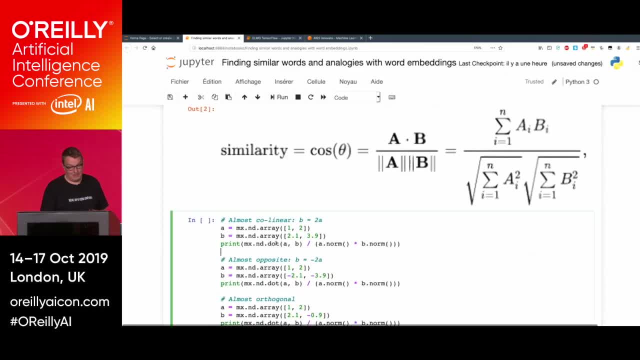 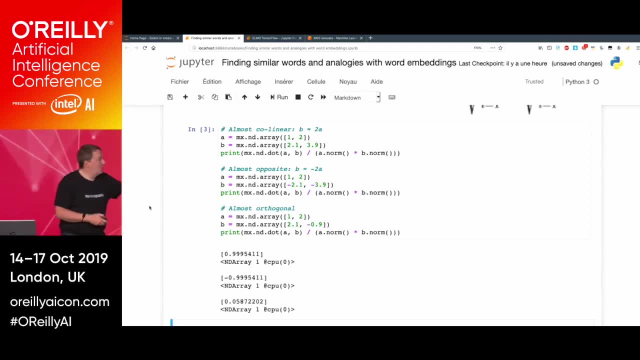 Okay, so here's an example if you're not convinced. Okay, so B is about twice A. Oops, yeah, so the cosine similarity is very close to one. In the second example, B is close to one. B is close to minus two A. 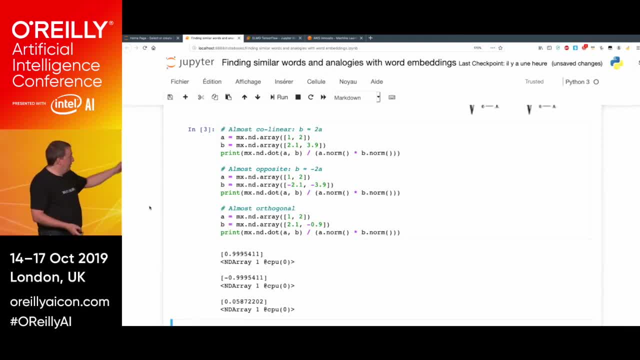 So cosine similarity is close to minus one. And in the third example A and B are almost orthogonal, So cosine similarity is close to zero. Okay, so it's nothing weird. Okay, plus one means similar, minus one means different Opposites. I should say: 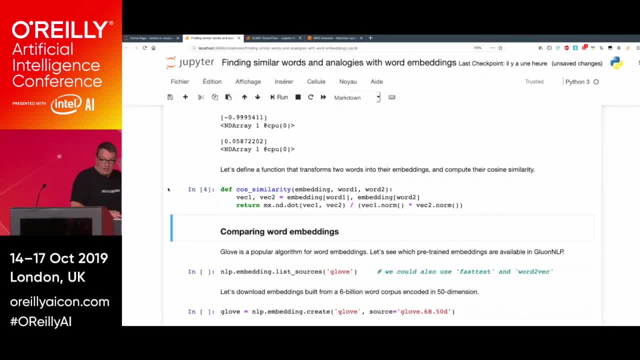 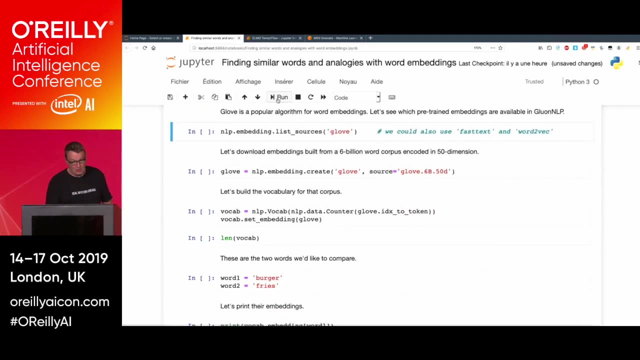 So let's define a simple function that will take a collection of embeddings and two text words, extract the embeddings for the two words and then compute the cosine similarity for those two vectors. Okay, All right. so now I need embeddings, So I'm gonna grab, I'm gonna look at. 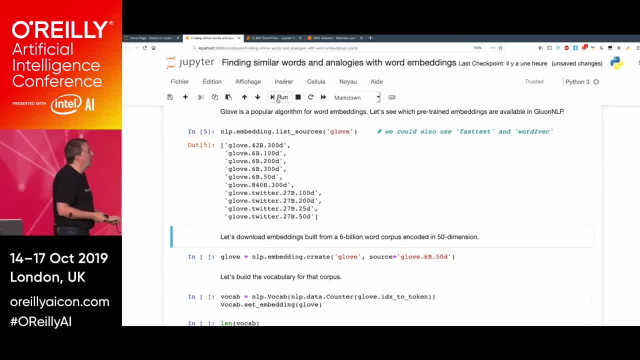 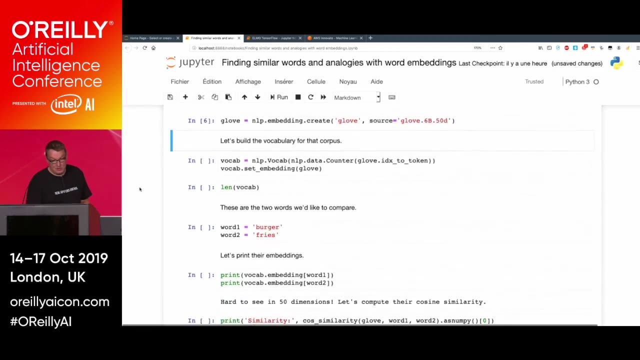 what Gluon NLP provides. I'd like to use Glove here So I can see all those collections of embeddings are available. I'm going to grab the small one. I already downloaded it. so it's six billion tokens and 50 dimensions. 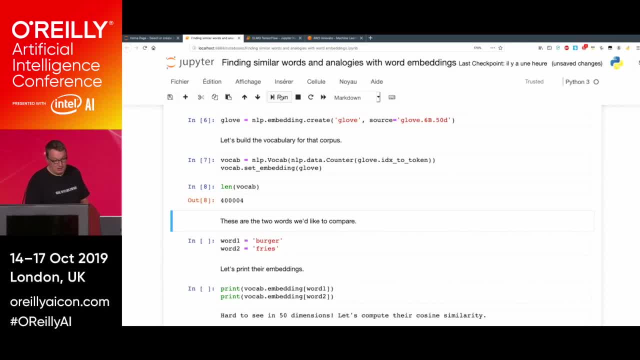 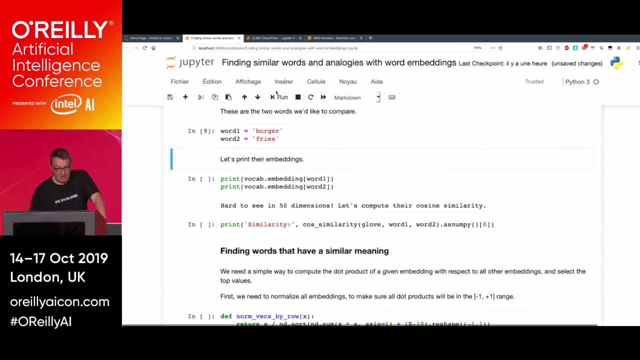 I can see how many words this actually means. So it's about 400,000 words in the vocabulary. Okay, so not huge, but it should be enough. So now let's try to compare burger and fries. Okay, so we can print their embeddings, of course. 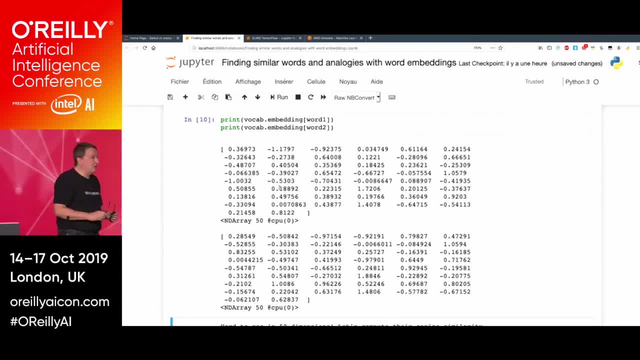 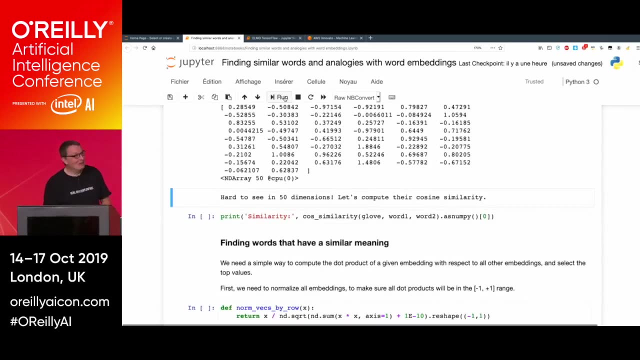 And no surprise, you get to 50 dimension vectors. So now you can compute in your head the cosine similarity, because you guys are better at math than I am. Right, Okay, who's got the results? Ah, come on Good. 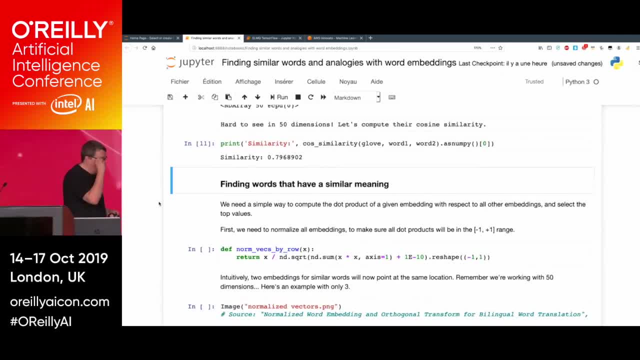 So it's hard to see in 50 dimensions right, We can use our function and it says the cosine similarity is 0.8.. So pretty close. So it means burger and fries are used close to one another in the same context. 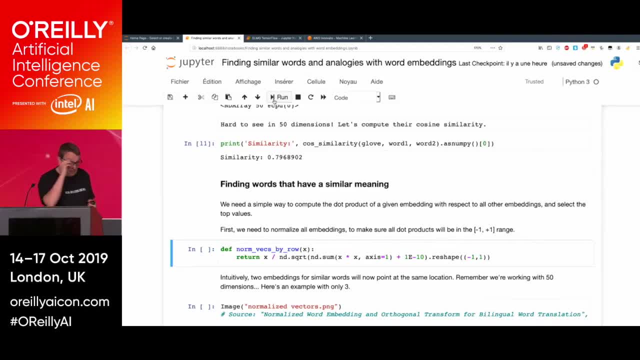 So now we could try: okay, let's give a word and find the top case similar words. So to make sure all vectors have the same length, I need to normalize them. Okay, so that's the best intuition I can come up with. 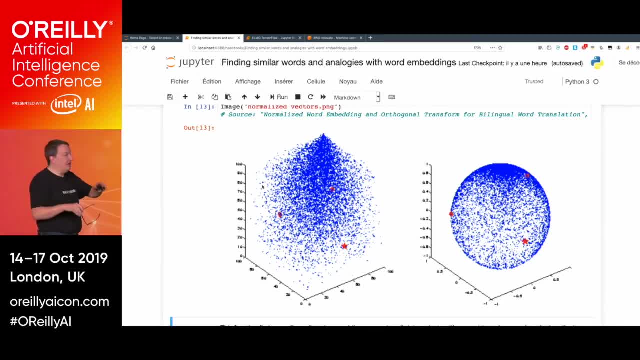 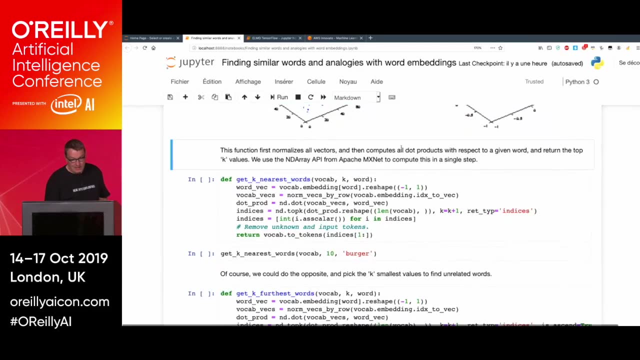 So you have 400,000 vectors with different lengths and you want them to be normalized because, of course, if you compute dot products, they should all be between minus one and one. Okay, so we normalize all the vectors with a simple function here. 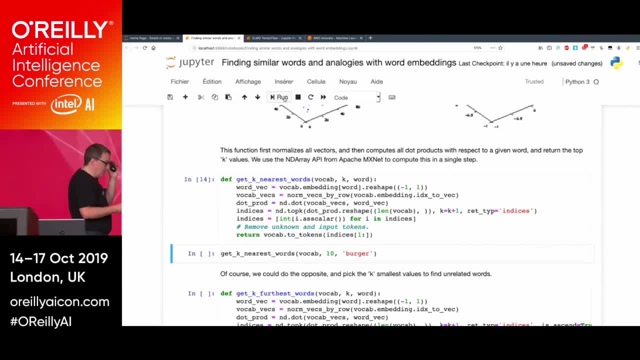 And then what this function does is really. it's a function It really takes. it takes a word, finds its embedding, computes all the normalized dot products between this embedding and the 400,000 ones, and then it finds the top K values and returns them. 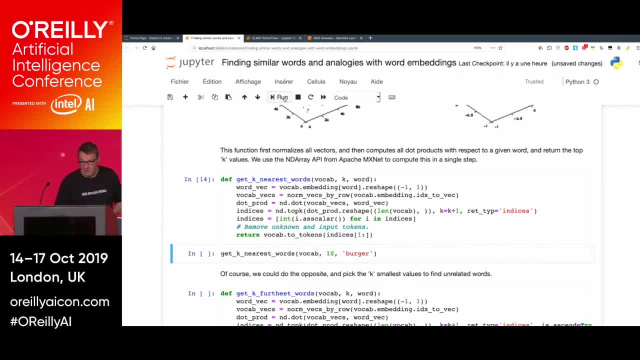 Okay, So this is 400,000 dot products in one go, and I'm using the MXNet ND array API to do this, which is close to NumBy, except, of course, you can run it in GPUs if you want to, and you can distribute it. 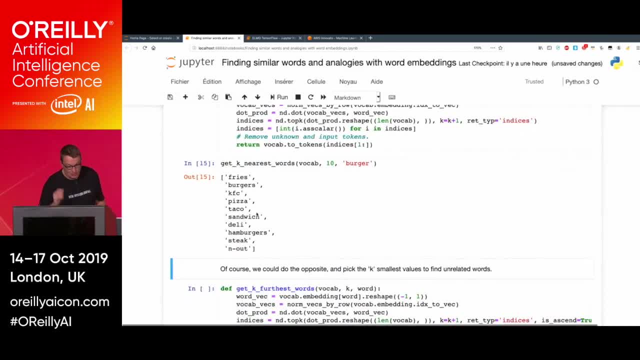 Okay, so let's find the 10 words that are the 10 vectors that are closest to burger. So fries, burgers, KFC pizza, tacos, sandwich, deli, hamburgers, stack and out, which might be a mistake. 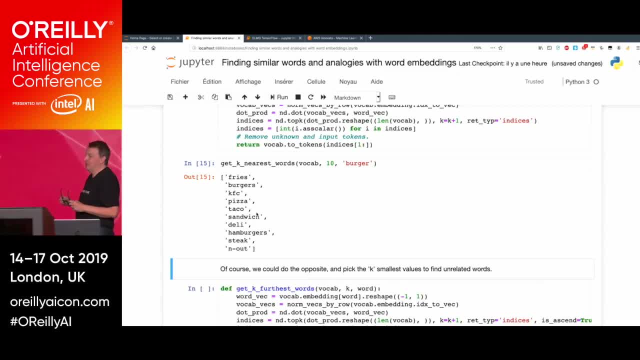 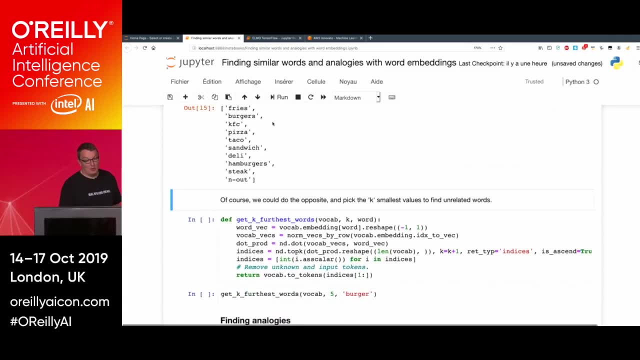 because there's this burger chain in the US called in and out, and I'm guessing this is what it is. So, okay, these are the close words. So of course, we could do the opposite And find the small the most different words. 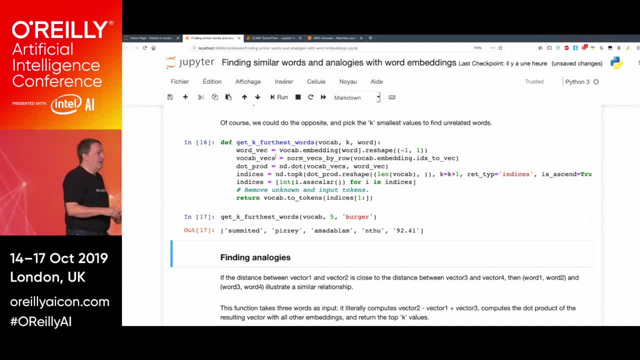 So it looks like in our six billion token vocabulary. those words, whatever they mean, sounds like Ktulu stuff or I don't know. What is this stuff Summited? Is that a word? It is a word, Okay, all right. 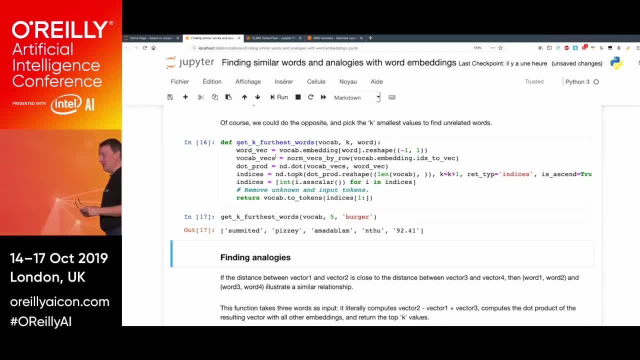 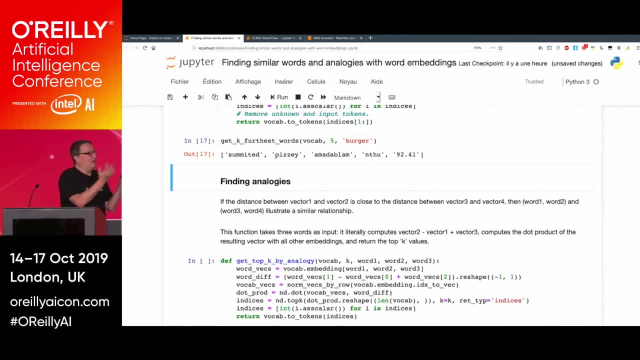 Pizza? no, I have no idea, Okay. Okay, So these things are never used in the same context as burgers, so we can ignore them. All right. okay, so you can find similarities. Now we wanna find analogies, okay. 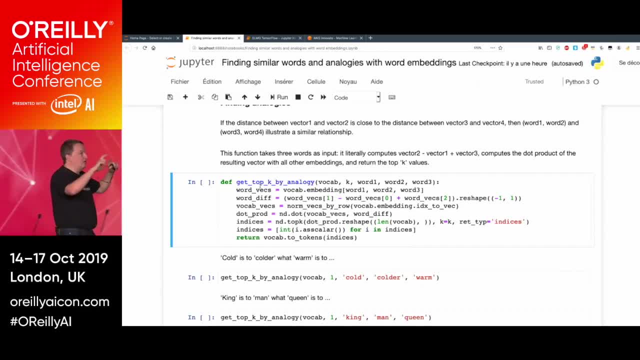 So remember what we said. you know, pairs of words that illustrate the same concept should be close. So what we're doing here is we're pressing three words, finding their embeddings, and then we're literally doing word one minus word zero plus word two. okay, 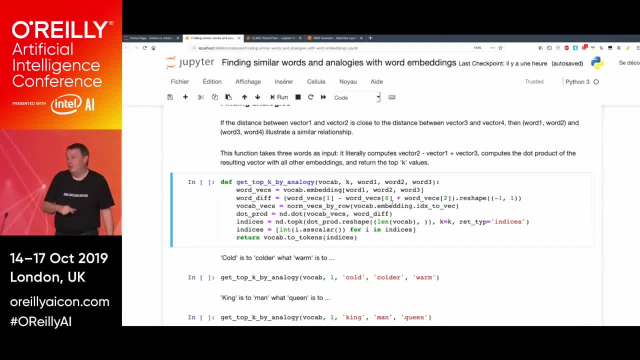 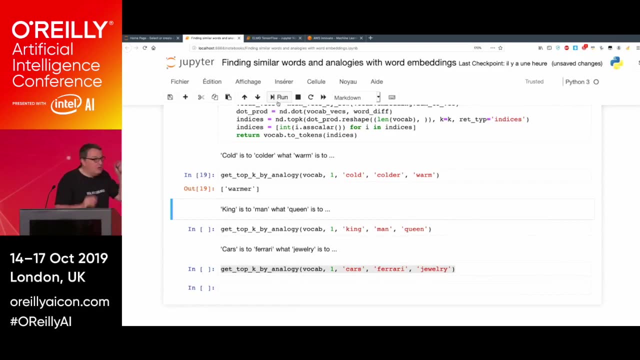 So computing the distance between the first pair of words and then adding the third vector, and hopefully that points to a fourth vector. okay, And now we can do this. so cold is to colder, what warm is to warmer? okay, The closest vector to cold, minus colder, plus warm is warmer. 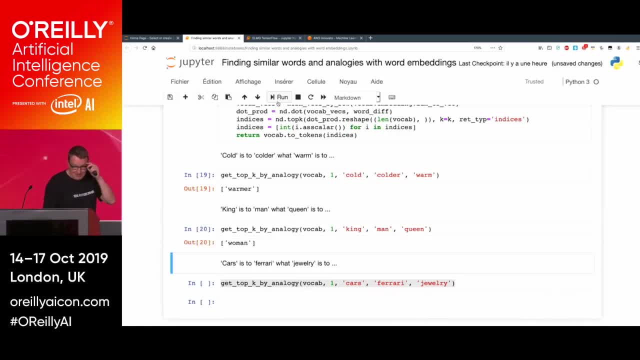 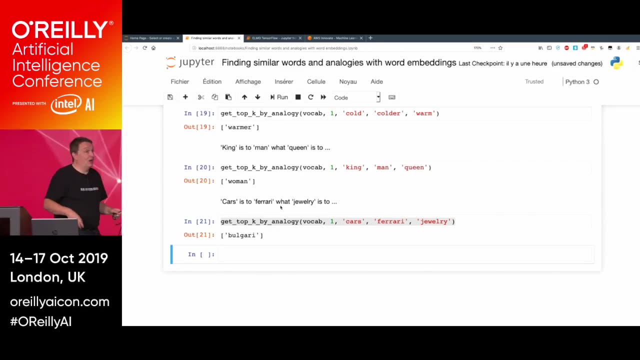 And the example that I would never believe with my own eyes until I saw it. yes, king minus man plus woman is equal to queen. so this is not fake. And cars are to Ferrari. what jewelry is to Bulgari, I'll let you judge, but it makes sense. 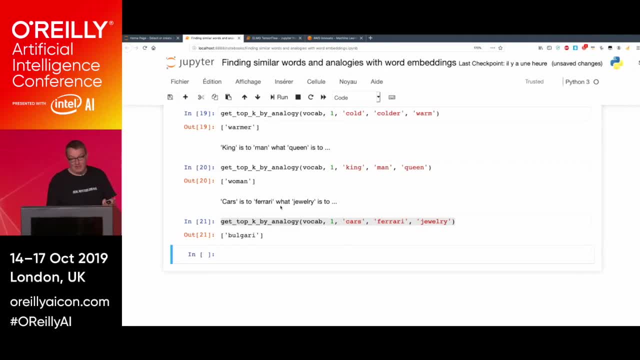 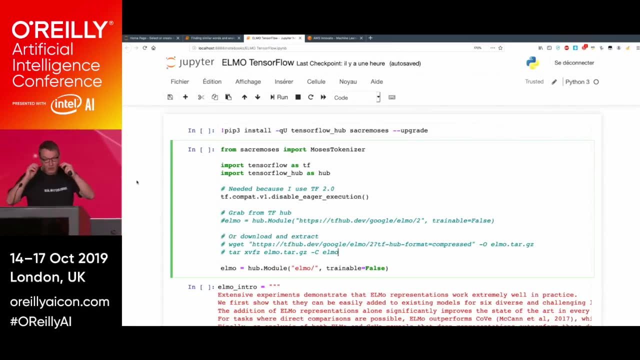 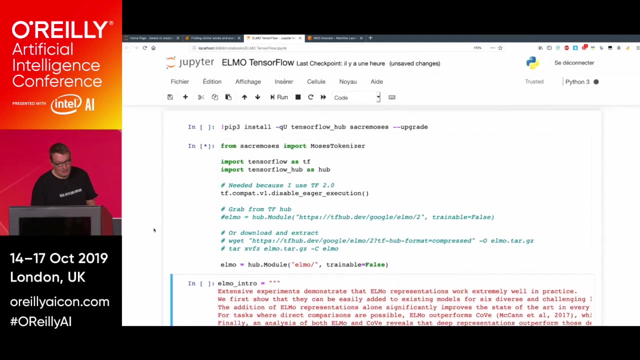 I mean, it's not a stupid answer, So you can find those analogies Okay. final example: I want to show you Elmo So you can download it from the TensorFlow Hub if you want, or you can download it locally, which I've done. 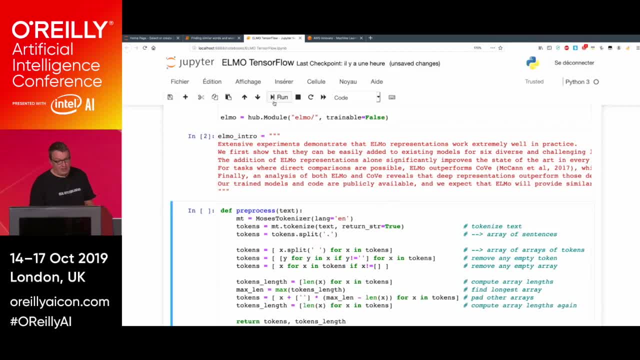 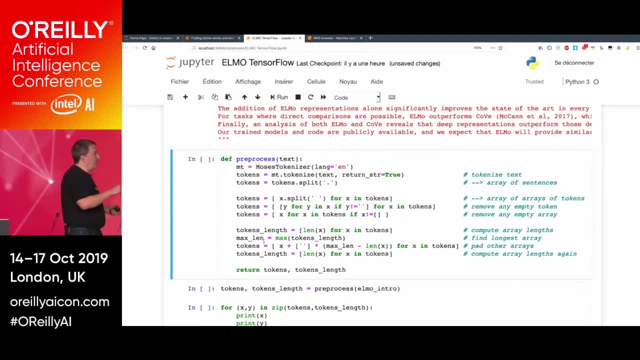 Yes, okay, so I can load Elmo. take some text from the Elmo article and I need to pre-process it. So, in a sense, what we're doing here is we want to split each sentence into a specific array, We want to tokenize everything. 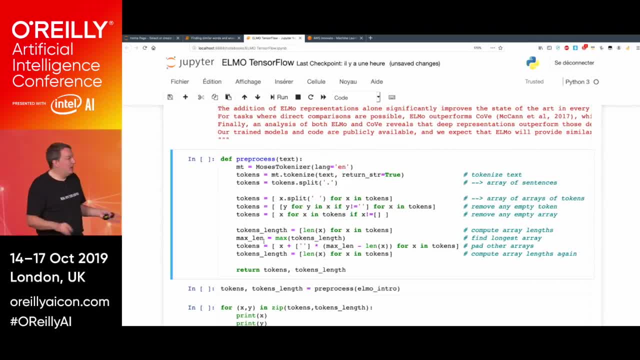 so make sure everything is spaced, separated, Want to remove any empty arrays, any empty tokens, And we need to compute the length of the longest sentence in here and we want to pad all the other sentences to the same length. Okay, that's what Elmo expects. 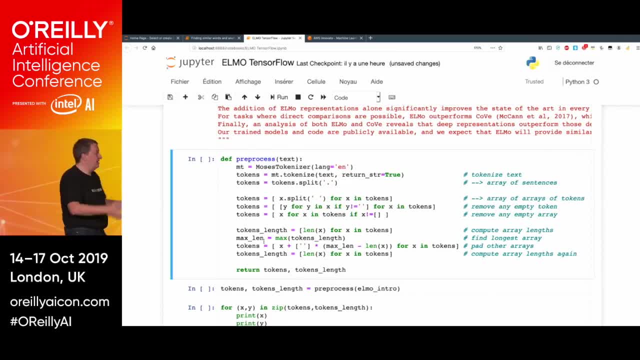 Okay, so it needs. the tensor that you're passing to Elmo needs to be correct. so all those space separated things need to have the same length and you might use padding for that. Okay, so let's not. and yes, God bless Python. 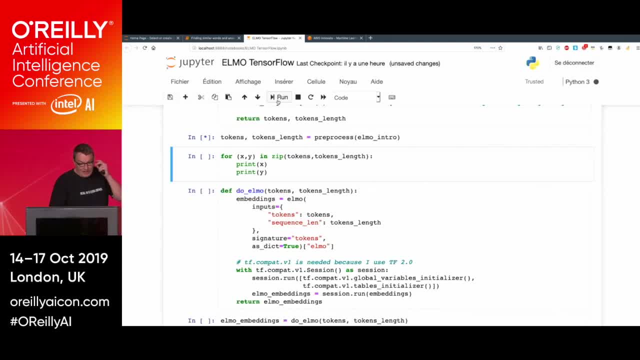 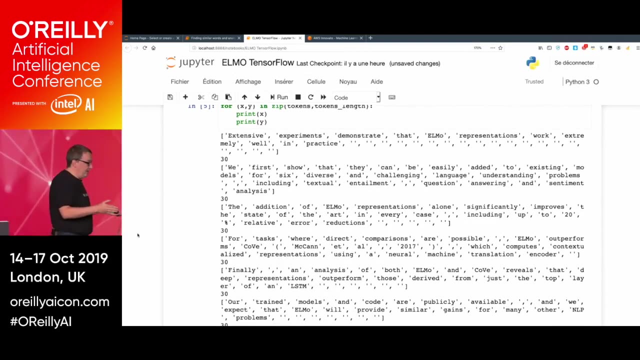 Right at scale. of course, you would not do it like this, So I can pre-process my text. Gonna take a few seconds and this is what it looks like. Okay, so the input is an array of arrays. Okay, each array is a space separated token sentence. 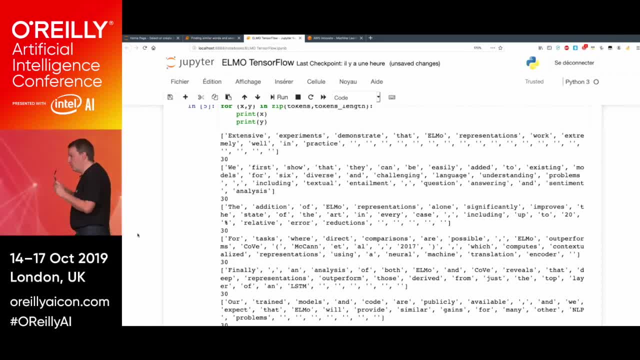 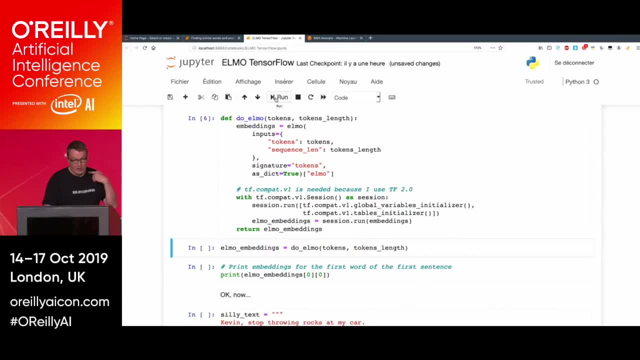 padded to the length of the maximum sentence here, which is 30.. All right, make sense. Okay, and now we can just pass that stuff to Elmo And I'm using. I have TensorFlow 2.0 installed here, which is why I need to have all the compact stuff. 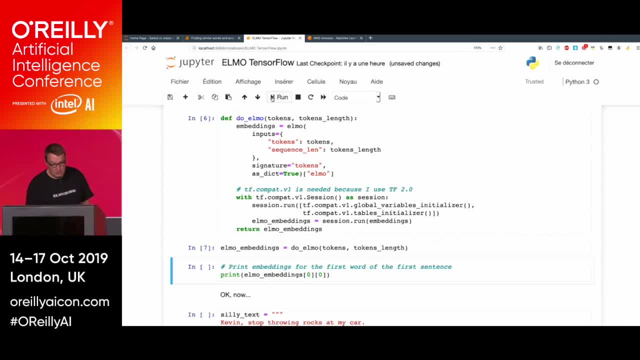 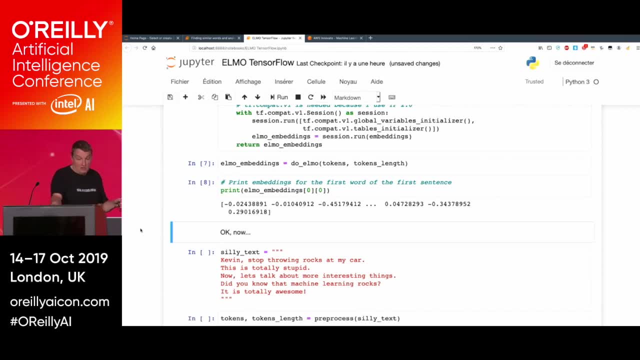 if you're using TF1X, then you could do away with that. And if I'm curious what the embedding is for the first word in the first sentence, okay, here it is Okay. so, as you can see, I need the model to predict. 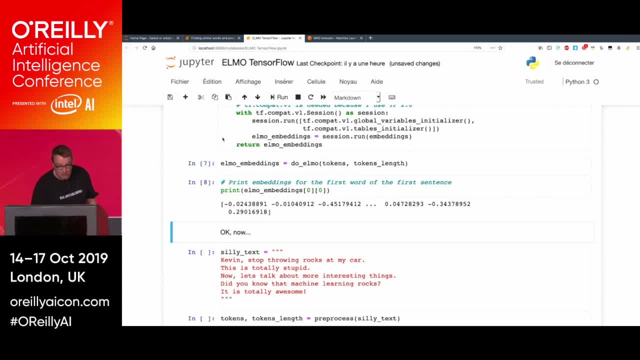 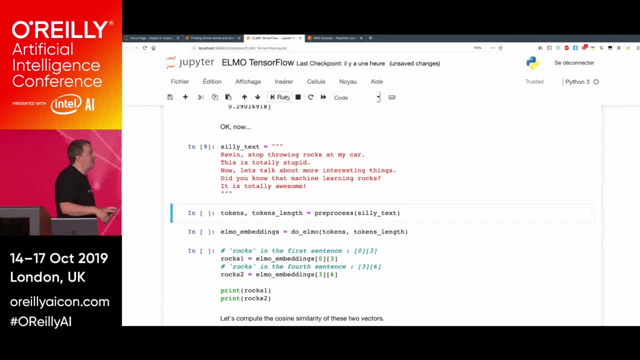 those embeddings and of course, I want to do this right. Kevin, stop throwing rocks at my cursor. he's stupid. Now let's talk about interesting things. Did you know that machine learning rocks? It's totally awesome. Two completely different uses of the word rocks.